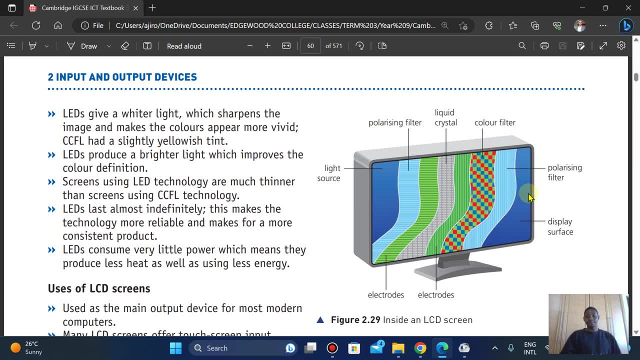 this is a good example of what i'm talking about. right, you can see the backlight right there, with the led of different colors, and that makes your, that makes the the um, the brightness, um, the constructs of your tv to be of optimal display. the led gives a whiter light which sharpens the. 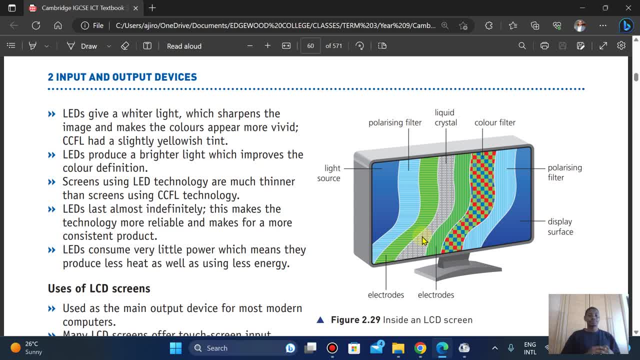 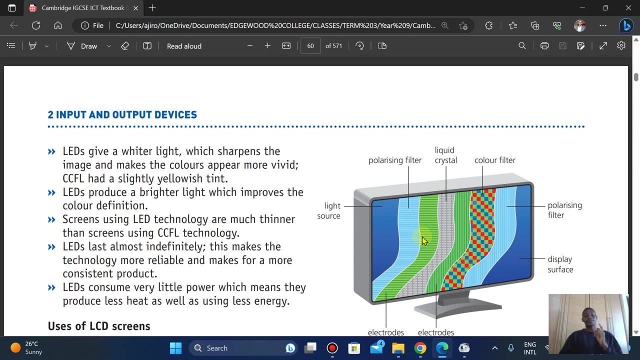 image and makes the color appear more vivid. um. the led produces a brighter light, which improves color definition. screens using led technology are more thinner than screens using the dc, dc, um, cfl, right, and if you wonder what they are, i just said it right here: they are the cooled 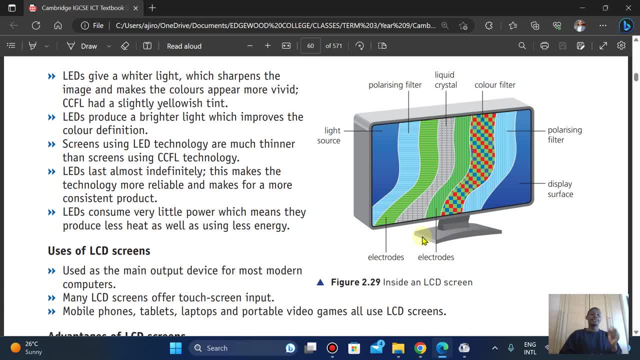 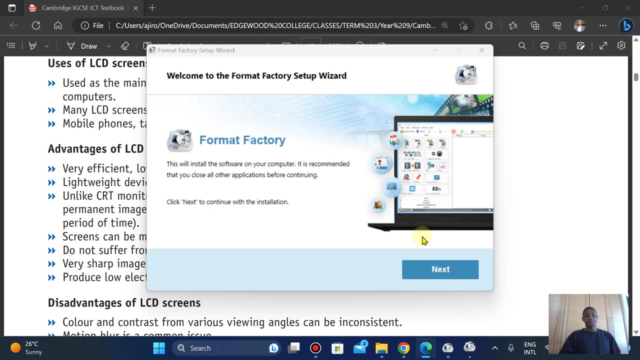 cartofluorescent lamp led last almost indefinitely. this makes technology more reliable, makes for a more consistent product. led consume very little power, which means they produce less heat as well as using the less energy. now, quickly, let's talk about the users. their users are two devices. 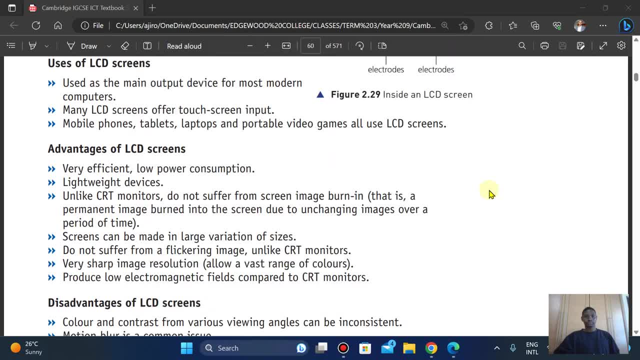 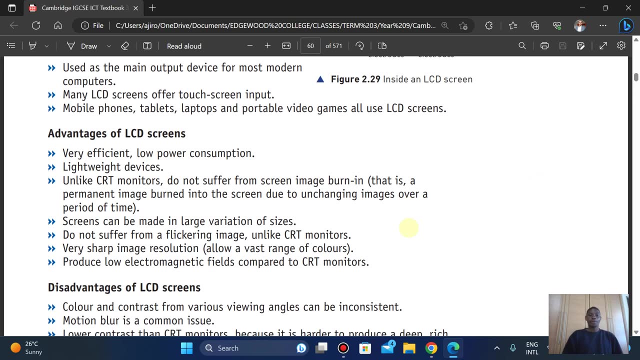 which is for more most modern computers. many lcd screens offer a touchscreen input. you can touch on them. but there's mobile phones, tablets, laptops, portable video games. all use the lcd screens. advantages: very efficient, low power consumption, lightweights. unlike the CLT, they don't suffer from screen burning. 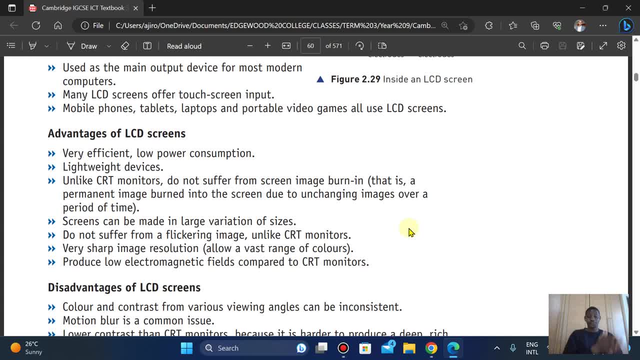 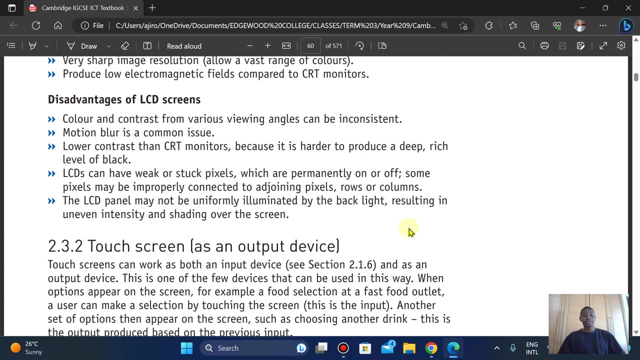 screens can be made a large variations of sizes do not suffer from a flicker screen, unlike we had in CLT. very sharp image resolutions produce low electromagnetic field compared to the CLT monitors. okay. disadvantage on the other end could be color and construct from various viewing angle can be. 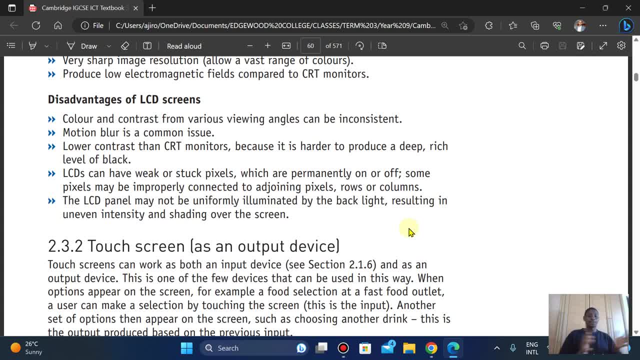 inconsistent, unlike the CLT that you know you can actually view from those angles. motion blur is somewhat a common issue. okay, let the low construct than CLT monitor because it's harder to produce a deep reach level of black. okay, LEDs can have weak or stock pixels which are permanently on or off. okay, the LCD. 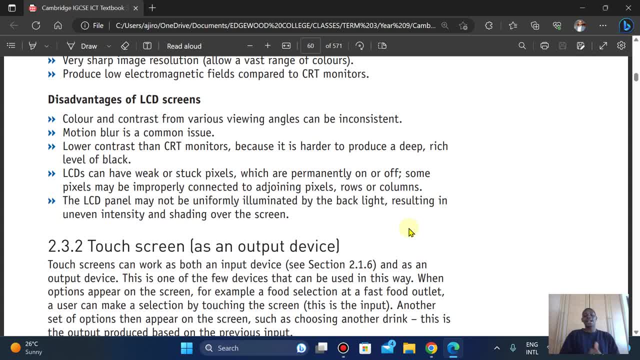 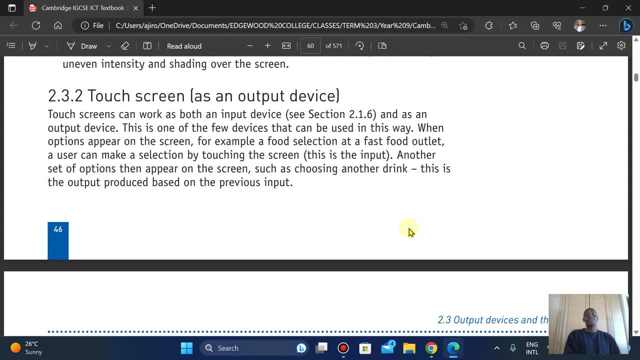 panels may not be uniformly illuminated by the backlight. okay, all right, let's talk about the touch screens. touch screens were looking at it as an output device. okay, now, this is one of the few devices that can be used in this way. okay, when options appears on the screen, for example, if food selection at a fast food outlet a user can make. 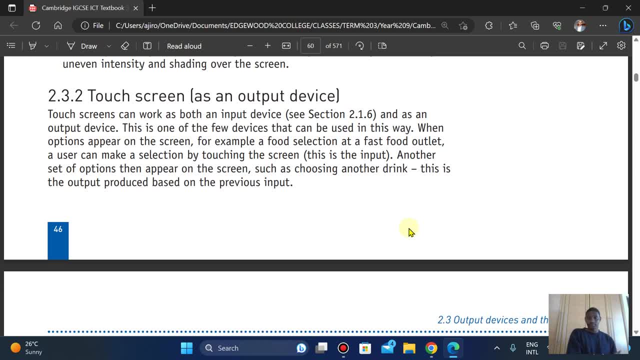 selection by touching screen. now, this is impute. we've talked about an impute. another set of option then appears on the screen, such as choosing another drink. this is the output produced based on the previous impute. okay, now use of the touch screen. now use of the touch screen. 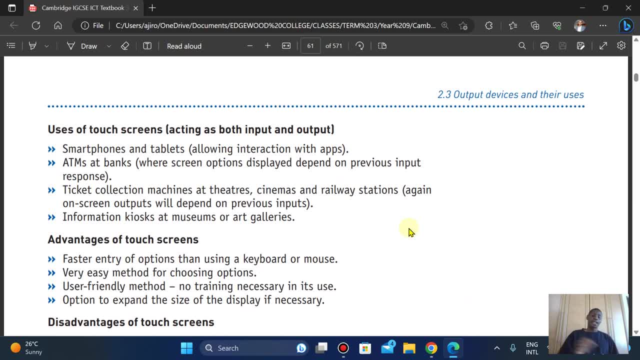 is acting as both imputes and output okay, so, looking at it, uses both of the input and output. is your smartphones and tablet okay, which allows you to interact with applications? ATMs at bank, where the screen option display- this bit depends on the previous impute- ticket collection machines at theater, cinemas and railway. 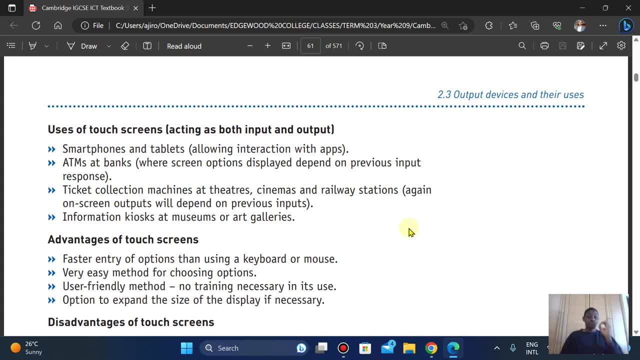 stations, information queues at mocks and art galleries. okay, so you can actually use the touch screens in this platforms now. advantages could be a faster entry of options using a keyboard or a mouse. it's very fast, very easy metal for choosing options. you don't have to get a. 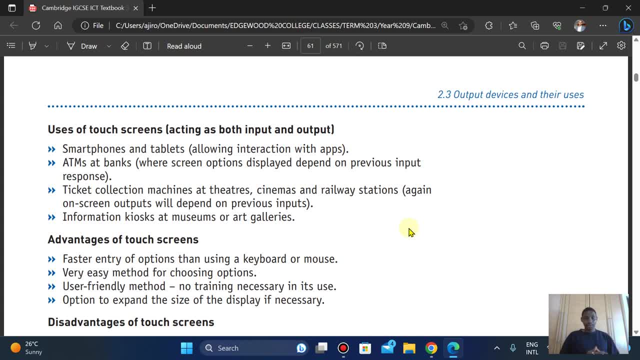 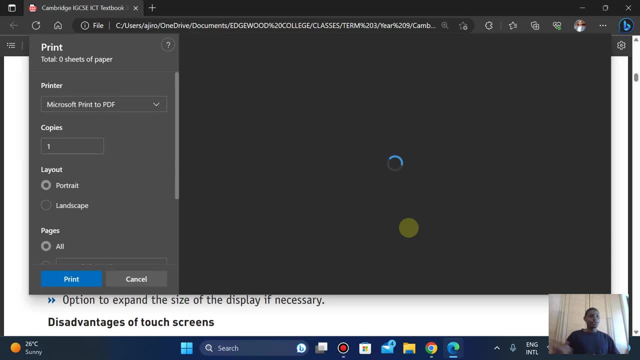 keyboard to choose. it's quite easy in the user-friendly method. simply mean that it's those. there's no training involved. all you have to do: you want to paint, you click here and then you print. you don't have to get a keyboard to screw your touchpad or to do this. no, no, no, you don't have to do that, okay. 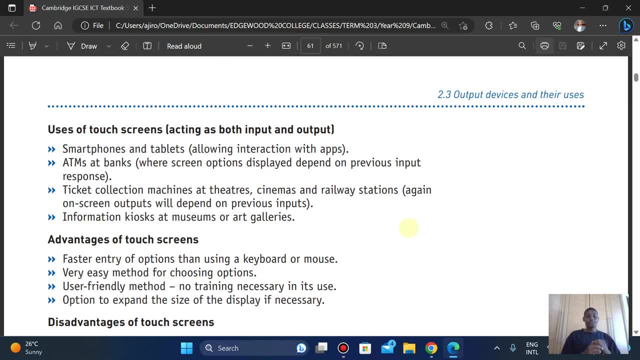 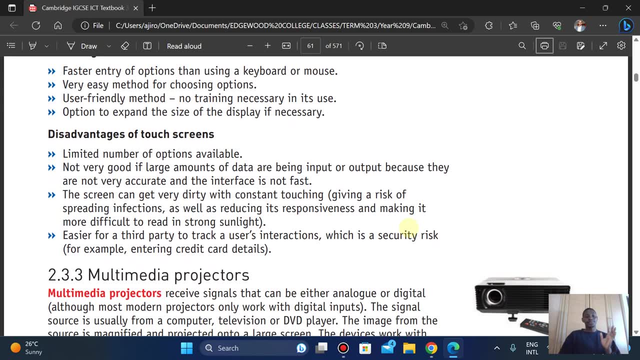 options to expand the size of display if necessary. there's an option to do that. however, disadvantages: there's a limited number of options available for you to do. not very good if large amount of data are being imputed or output being out because they are not very accurate and the interface is not fast. the screen. 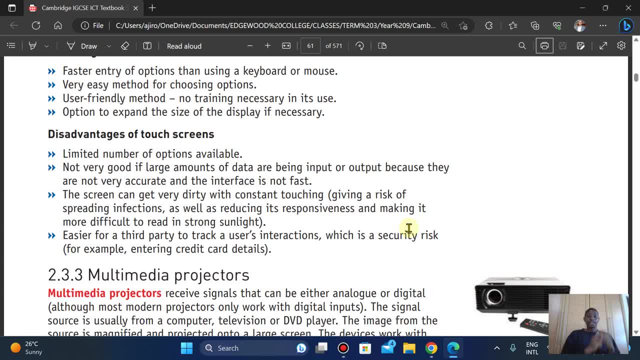 can get very dirty. that has to be part of the thing that comes to mind. okay, when did that constant touching? okay, giving a week's of, you know, reducing its responsiveness and making it difficult to read in strong sunlight. easier for a third party to track user interaction, which is a security mix. okay, credit card. 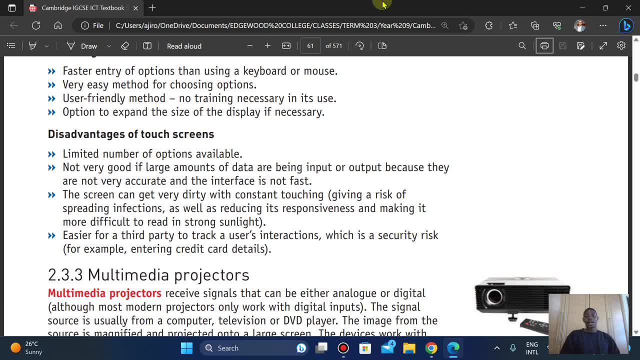 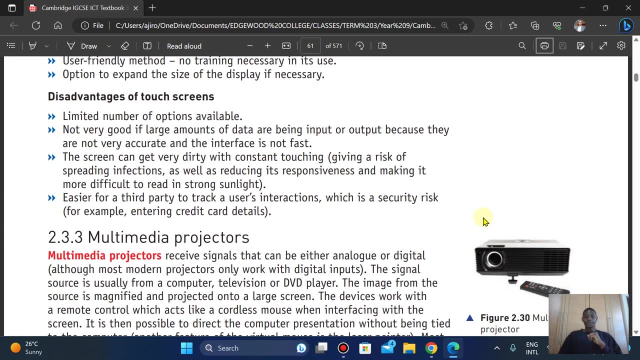 details, etc. etc. okay, now I want to believe you understood all this, but just in case you don't, please, you can always post back in. you know, go back in, come back again and to get more understanding on that. okay, multi media predictors, I want to believe you guys have seen a projectile, right. so 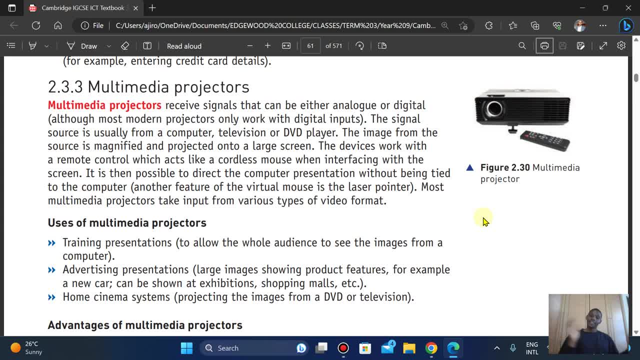 the projector received signals that can be either analog or digital in nature. okay, now, what this simply means is the signal source is usually from a computer, probably from a television, television or a DVD player. now, the image from the source is then magnified and projected onto a large screen. the devices work with a remote control. 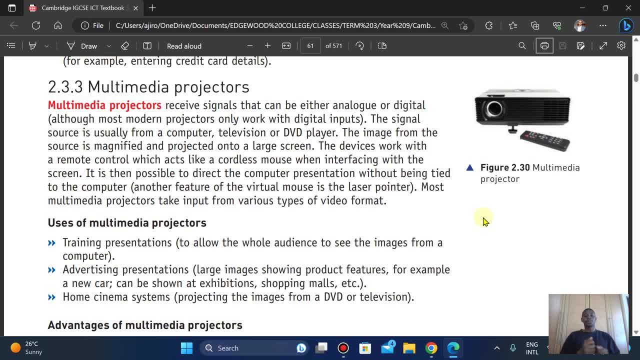 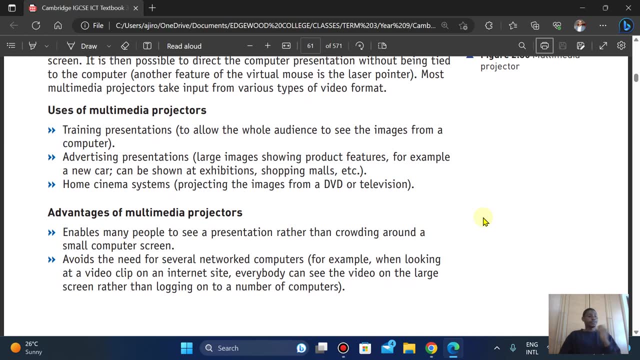 that acts like a cordless mouse, so it does remote control. that's like a conduct mouse when interfacing with the screen. now it is possible to direct the computer presentation without being tied to a computer. okay, now let's talk about users. you can use the projector when you're training making. 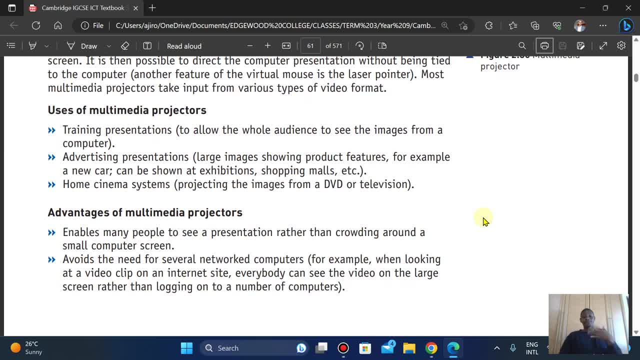 presentations on training, on various things you can do. advertising right um showing your product features um home cinemas, the mix of projectors right um protecting the image from dvds or televisions. advantages of multimedia protectors enable many people to see presentation rather than crowding around a small computer screen, avoiding the need for several network computers. 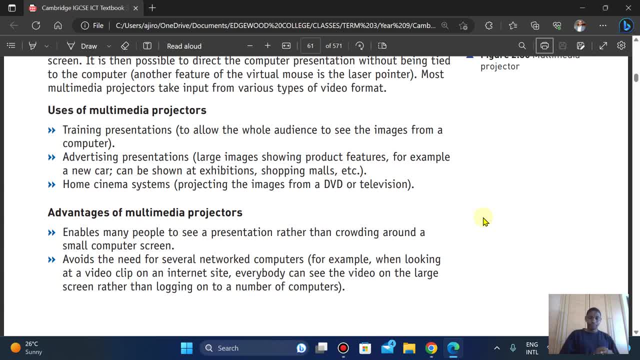 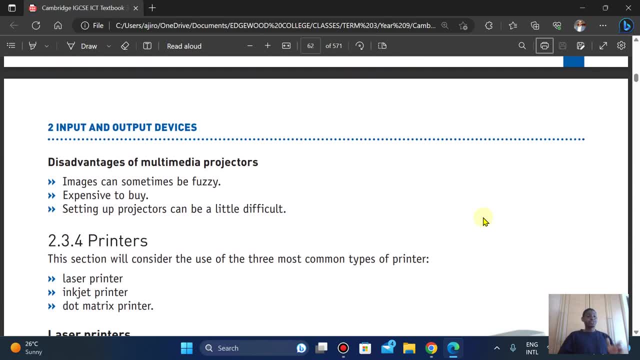 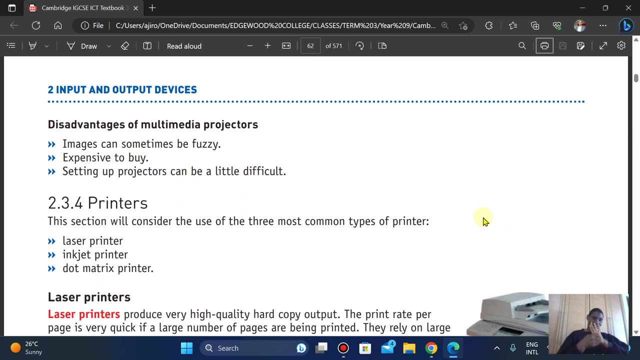 okay, we're looking at a video clip or an internet site. okay, so everybody can see what's on the last screen, right, whether they're just logging in and you're networking all the computers. disadvantage, on the other hand, is images can be sometimes, can be fuzzy sometimes, so you have to adjust it right. it can be fuzzy a little bit, blow, it can be fuzzy, so you. 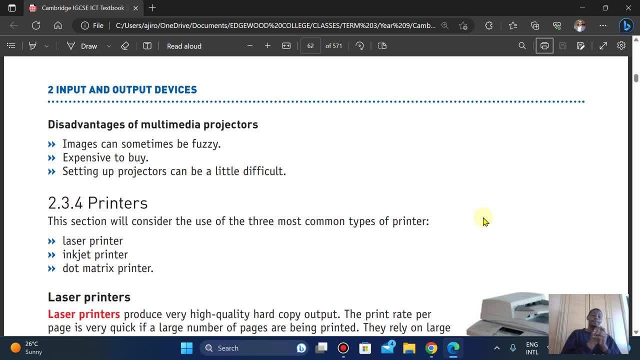 have to adjust it, but it's a disadvantage if you want to look at it and projectors are not easy to buy. they're expensive and setting up a projector can be a little bit difficult. okay, you have to set up depending on where you want to place it. depending on where you want to place it, okay. 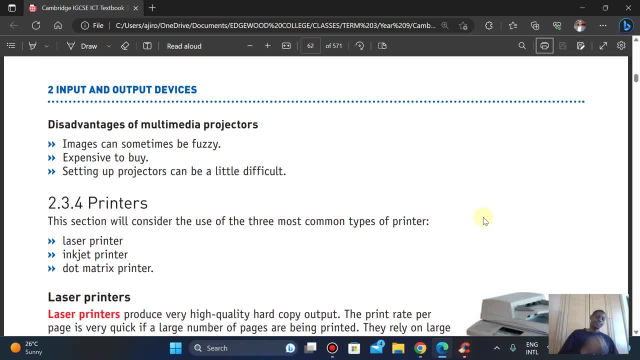 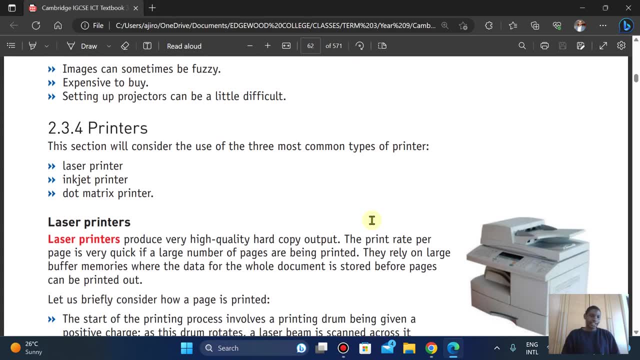 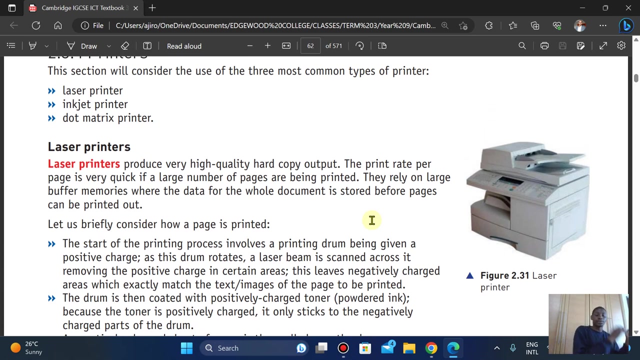 um, let's talk about printers now. this section covers. so we have the laser printers, inkjet printers, the dot metric printer. i'm just going to just compare the three of them and, um, because usually christians, they come on um advantage between one over the other. uh, but the first. the first thing you should understand about laser printer is: 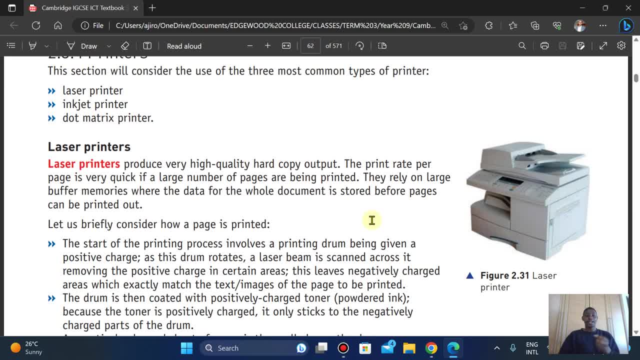 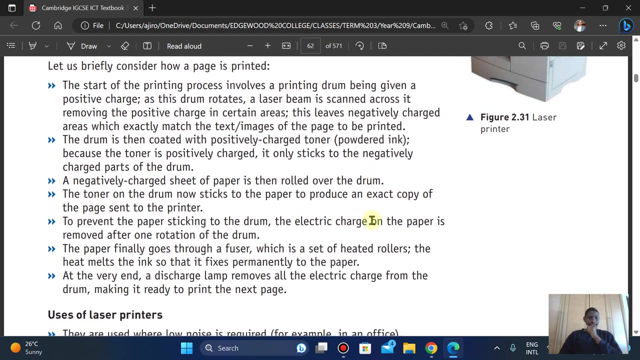 that they can produce a very high quality hard copy output- okay, um. they're very quick and in producing large numbers of pages- okay, and they also rely on what we call a large profile memory, where data for the whole document is stored before pgs can print it out- okay, um. another thing is that 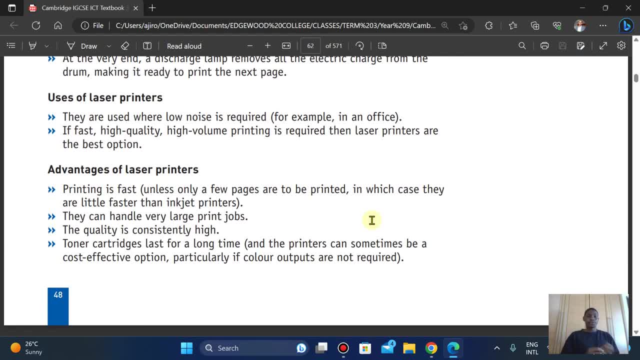 is the use of printers. They can be used. laser printers are used where low noise is required. If fast, high quality, high volume print is required, then laser printers are the best options. okay, Printing is fast. That's an advantage for laser printer. 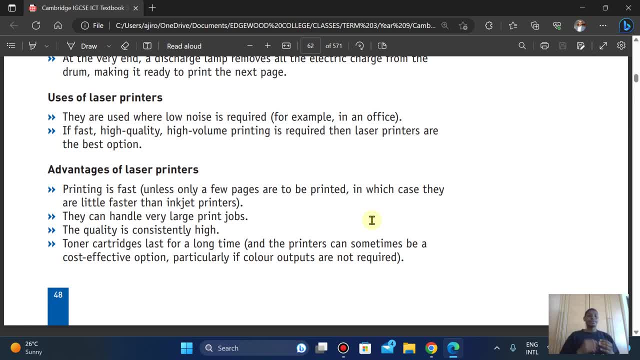 Printing is fast. okay. In which case they are very little. in which case they are a little faster than the inkjet printers. okay, They can handle very large print jobs. The quality is consistently high. okay, The toner cartridge they use lasts for a long time- okay, 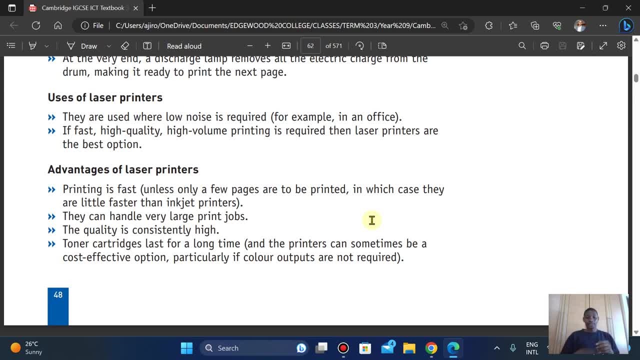 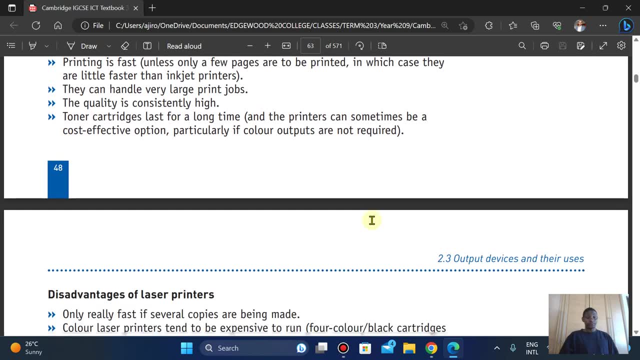 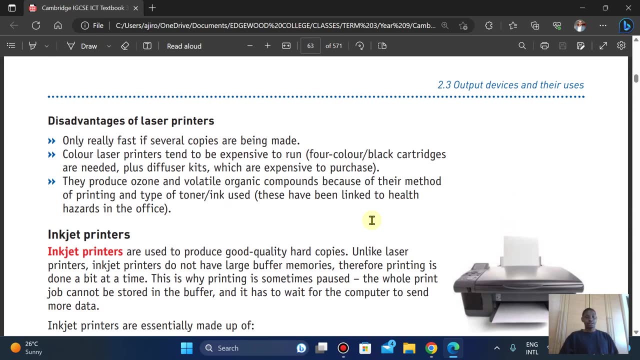 And yes, they can be cost effective. okay, Especially if color options are not required. But if color options are required, then they are very costly. Disadvantage: is that only really fast if several copies are being made? Okay, if you're printing one one. 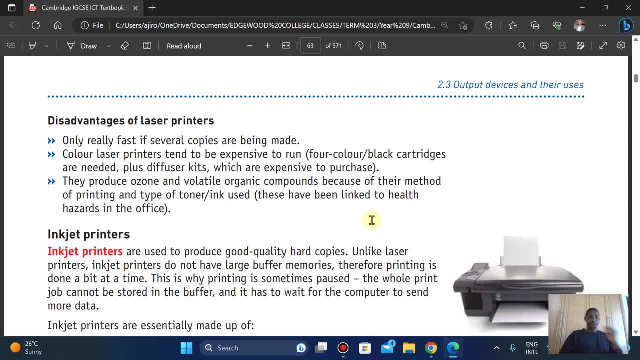 you're not going to need your. but if it's fast copies, this is really for printing fast copies. Color laser printer tend to be expensive too. I've talked about it as well. They produce ozone and volatile organic compounds because of their method of printing. 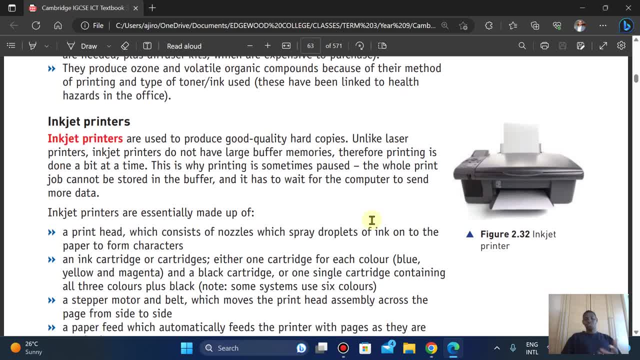 The inkjet printers, which is more like a home use printer. they produce good quality hard copies, right, Unlike the laser printers, right, They don't have large beep for memories, Therefore, printing is done one bit at a time In terms of quality printing. 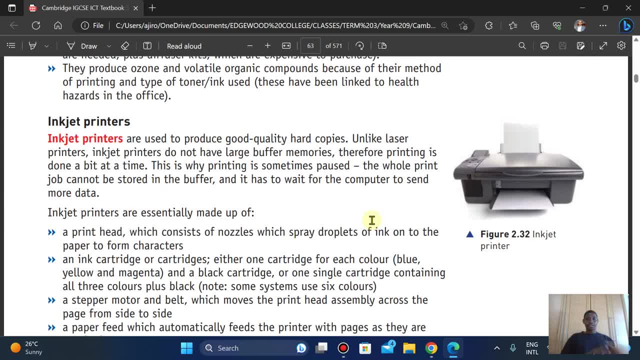 your inkjet printers is better than laser printers. okay, It's better than the laser printers, okay. Another thing is printing. like I said, printing is done one at a time, okay. That's why printing sometimes pause. The whole print job can not be stored in the boom. 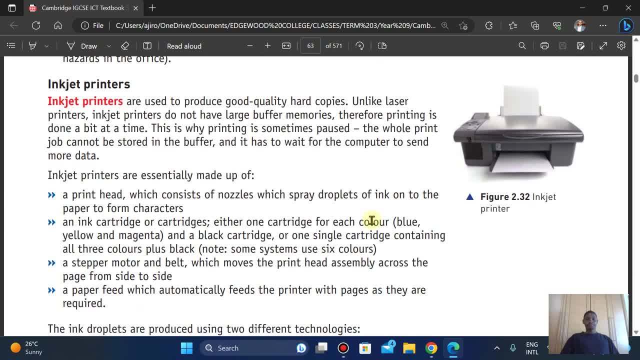 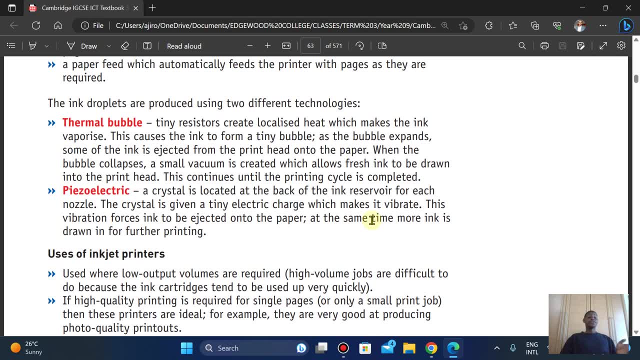 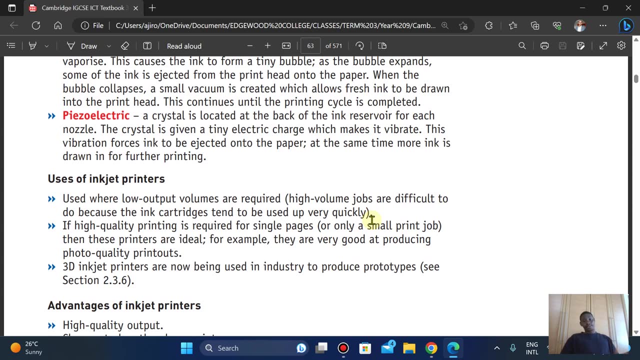 way for the computer to send in more data. okay, now, um, they are based on different technologies: the thermal bubble and the piezoelectric. okay, the use of the inkjet printers is that they use. they use where low output volumes are required. okay, they don't print high volumes, okay. 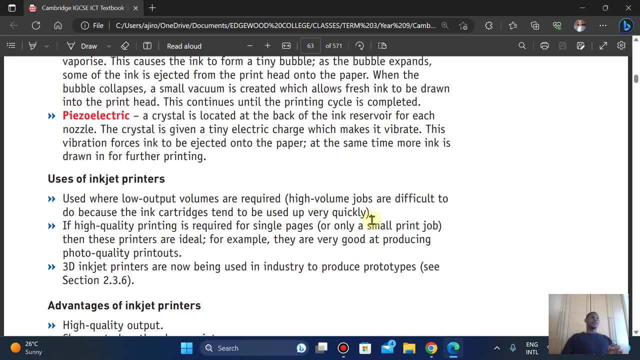 and this is because of the ink cartridge. okay, it's tend to be what used up very quickly. if high printing is required for a single page, then this printer's id. you want a high printing for a single page, right, a color printing. it has the photo quality. the inkjet printer is probably your best. 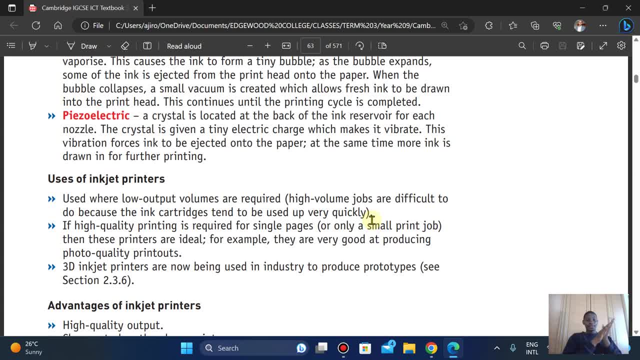 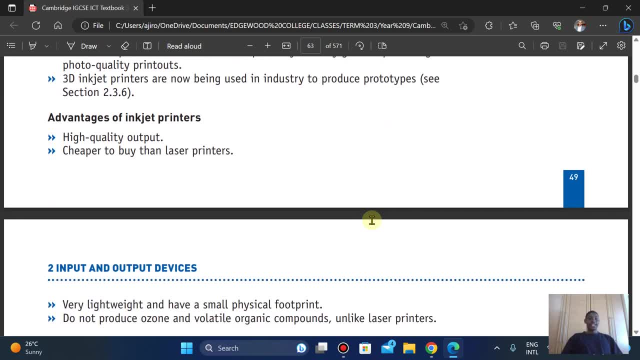 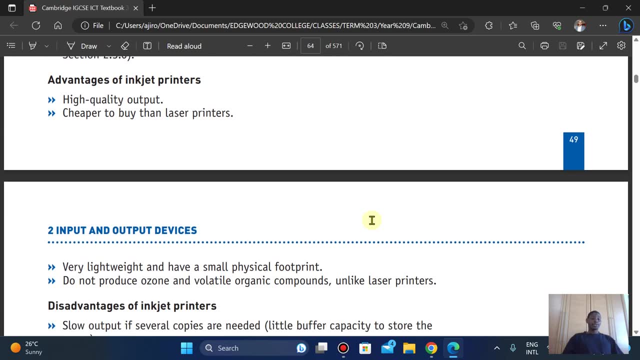 bet okay. um, the 3d inkjet printers are now being used in industry to produce prototypes. okay, we're going to look at that as well. okay, now advantages of the agent. the inkjet printers is high quality output cheaper to buy than laser printers. they are home use. um, they are very lightweight and have a small physical. 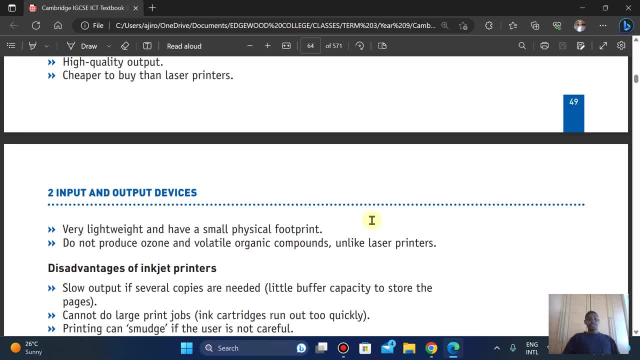 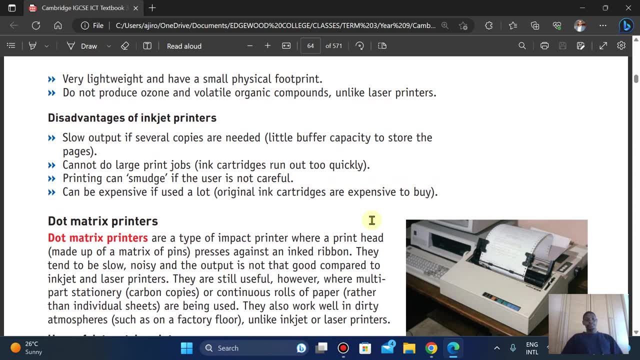 blueprint do not produce the ozone or volatic, volatile organic compounds. disadvantage is that um it slows output instead of copies are needed, so it's not ideal for printing. large copies cannot do large printing jobs. printing can smog if the users is not careful, so you have to be. 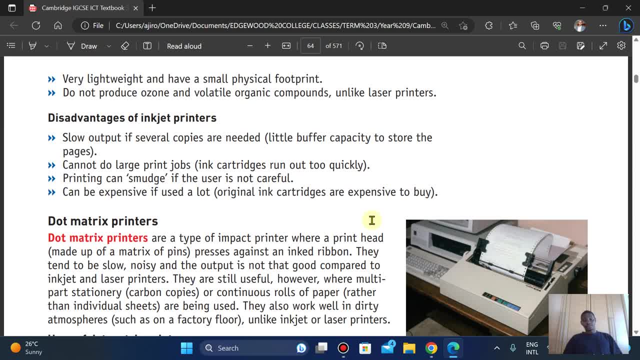 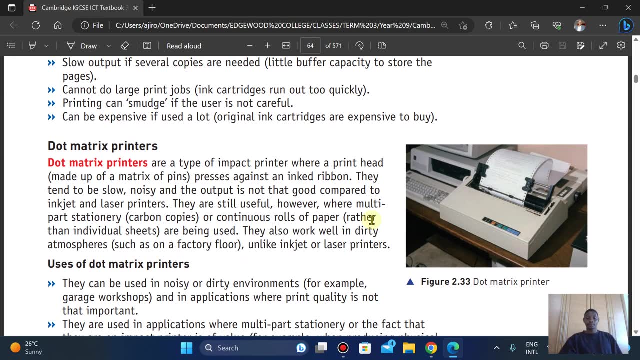 very careful when you print it. okay, it can be expensive if used a lot. talking about getting the inkjet cartridge right, another one is the dot metric printer. okay, where the print head is made up of what? um? okay, it's made up of your matrix of pins. right, it's pressed against an ink ribbon. okay. 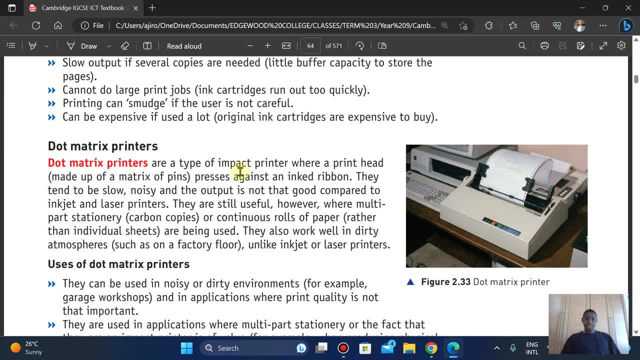 now. they tend to be slow, noisy and output is not good compared to the inkjet laser printer. you need to know the difference. okay, they tend to be slow, noisy and output is not good compared to the inkjet laser printer. they're still useful, however. they are multi-pass stationaries. right. rules of 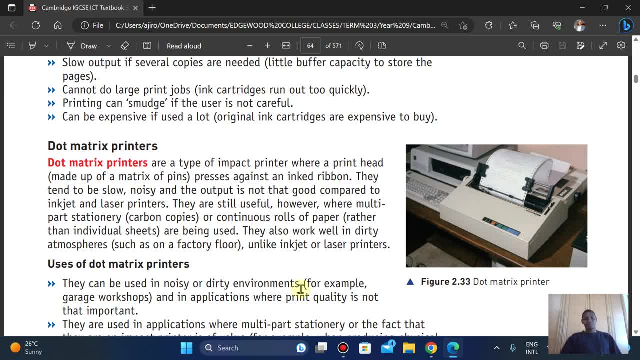 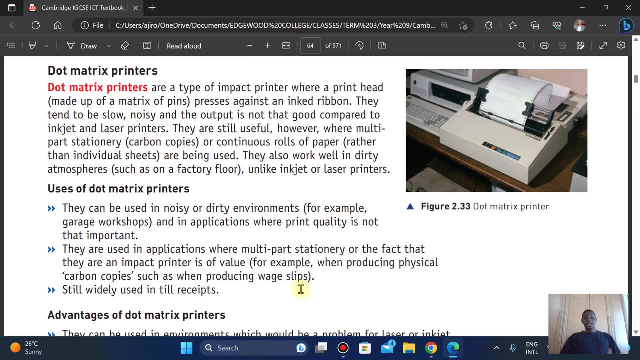 papers okay that have been used. they work well in dirty atmosphere such as factory floors, like your inkjet or lisa printers okay. they can be used in a noisy or data environment where the print quality is not that important. um, they are using applications where multi-party. 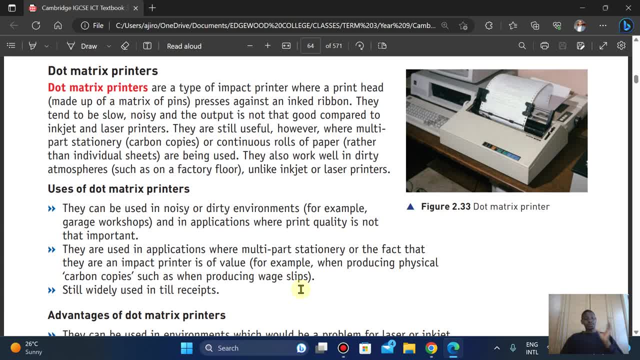 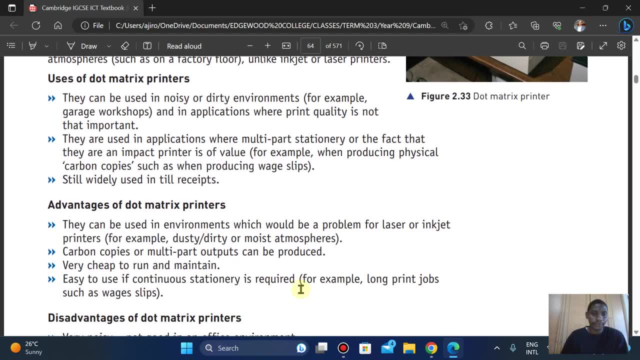 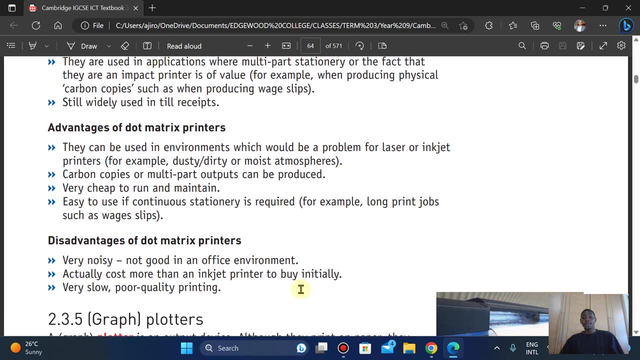 stationaries, or the fact that they can. their impact printers is of value. still widely used in steel receipts. okay, okay, um, they are used in environment where which will not- which would be a problem for laser or inkjet printers- okay, um, they can be used in that environment. that's because, for example, it's a dusty. 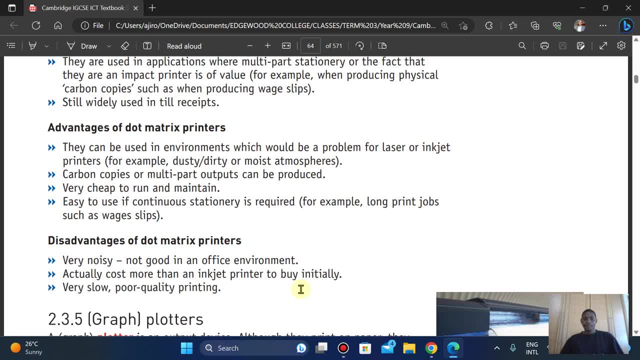 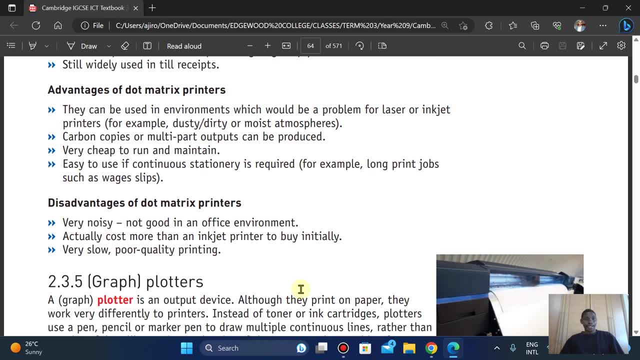 authentic environment: moisty, atmosphere. it's fine. carbon copies or multi-part outputs can be produced very cheap to run and maintain and, again, easy to use if continuous stationery is required. the survival that i had is noisy. it costs more than the inkjet printers to buy initially, it's very slow and it has a poor printing quality. the next one is a plotter. 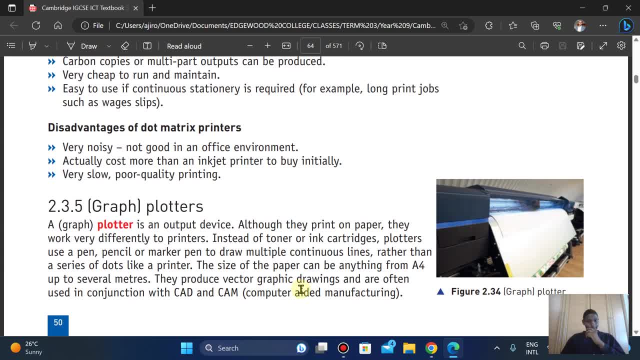 right. um, it's an active device: the print of people. they work very differently to printers. instead of tuners or ink cartridge, plotters is what we call a pen, pencil or marker to draw multiple lines rather than the series of dots, like the printers. now the size of the paper can be. 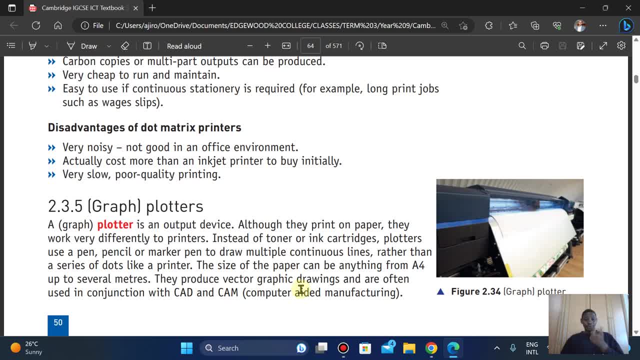 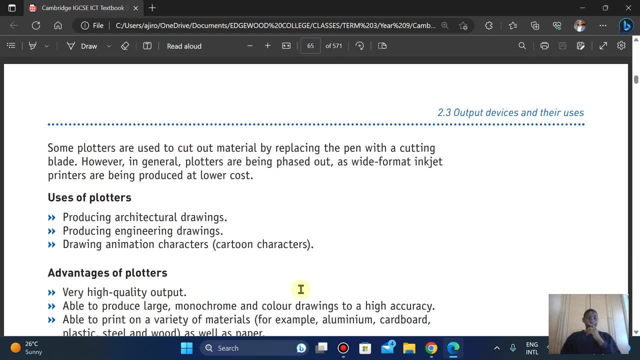 4 to 7 meters. they can produce what we call the vector graphic drawing and have to use the condition with your card or your cam. now, another thing is. one good use about the plotters is they are used for producing architectural drawings, engineering drawings, doing animation characters. 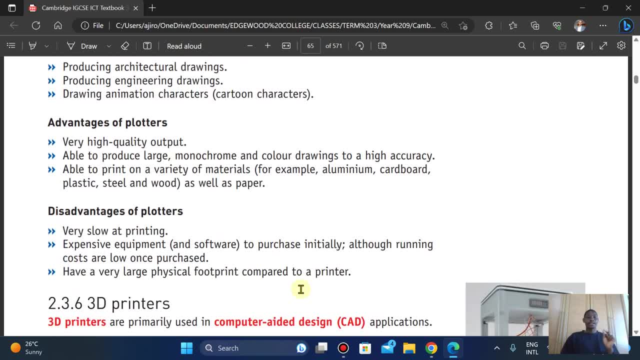 okay now they have very high um quality output. they're able to produce high monochrome and color drawing to a high accuracy. okay um able to print on varieties. they can print on a lot of material. they can put on cardboard, aluminium, plastic, steel, wood. that is the good. 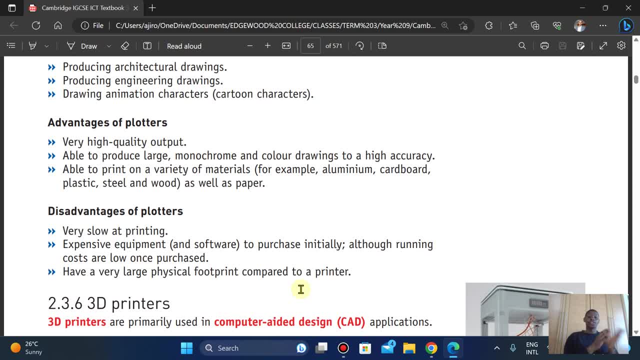 thing about this printer, unlike other printers that mix with just paper, they can print on anything. okay and um it's about- is that it is slow at printing. it takes time in printing. all right, this is expensive, okay equipment to purchase. okay, um, although the running costs are low once. 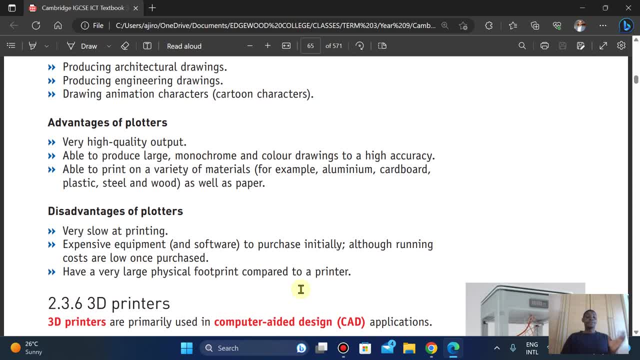 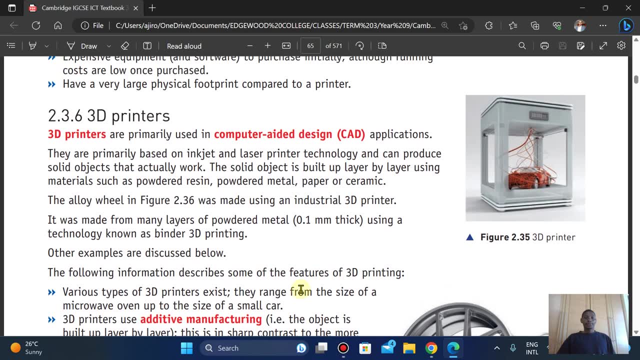 purchased, but it's expensive to purchase the initial cost. they have a very large physical footprint compared to a printer. now the next one is the 3d printers. now, the 3d printers are probably used in the computer either design applications, okay, and they are probably used with the inkjet and laser technology and they produce solid image that can. 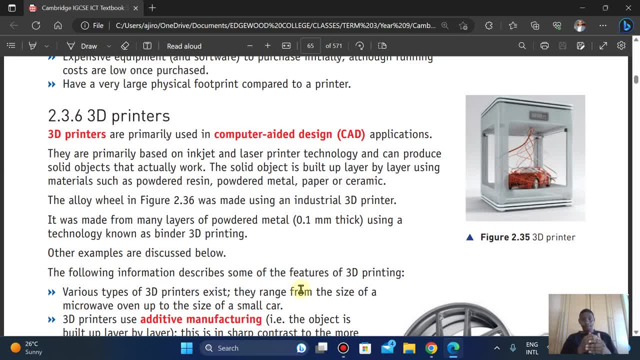 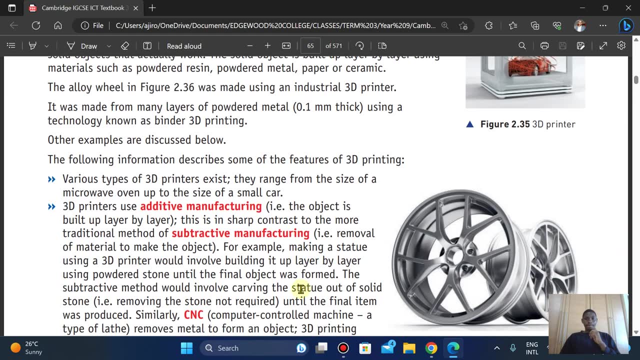 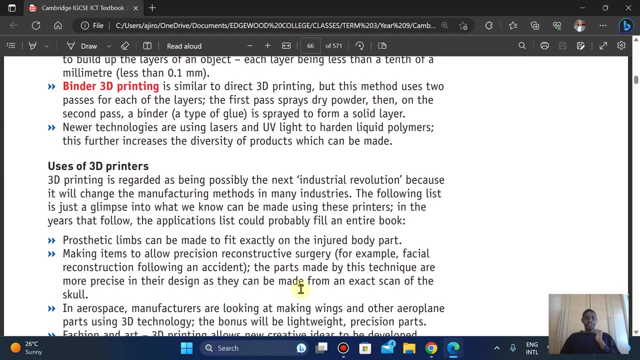 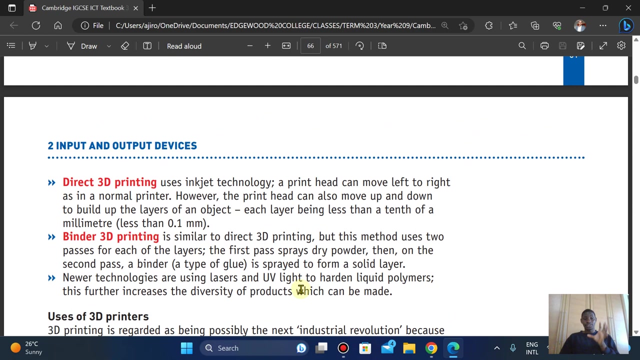 actually work okay, they print our prototypes okay, and this object is built layer by layer, using materials such as a lot of paper, ceramic, a lot of things to do that. um, now let's talk about the uses of these 3d printers. now, the use of the 3d printers is okay. just a quick one. um, we have different kinds of the 3d. 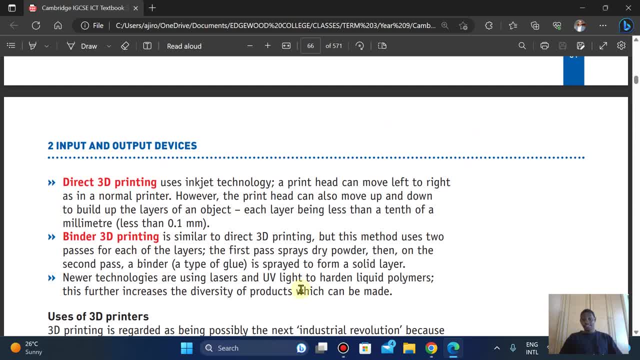 printers. we have the direct 3d printers. that uses the inkjet technologies. a printhead can move from left to right as in a normal printer. okay, um, we have the binder 3d printer, right, which is two passes for each of the layer. uh, the first place we drive spoiler, and then you know, you know the rest. 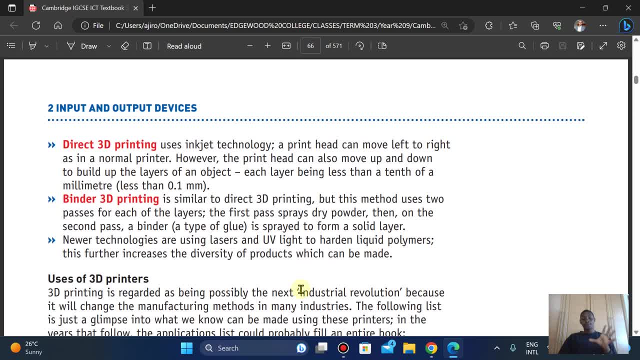 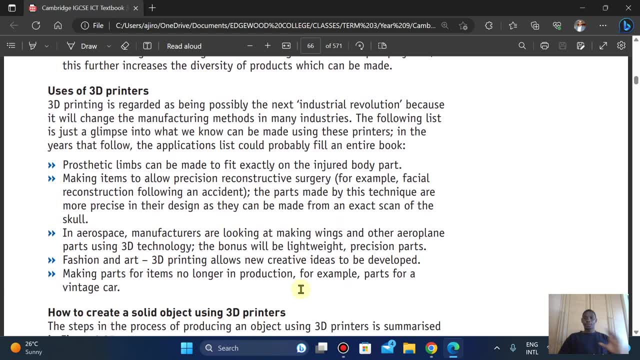 okay, um, although this is best explained using a video, okay, and probably um for students, i'm just going to drop a copy of a link of the video on the 3d printer so you can see this as it's working in real time. now uses is um for prosthetic limb can be made to fit exactly on the injured body part. 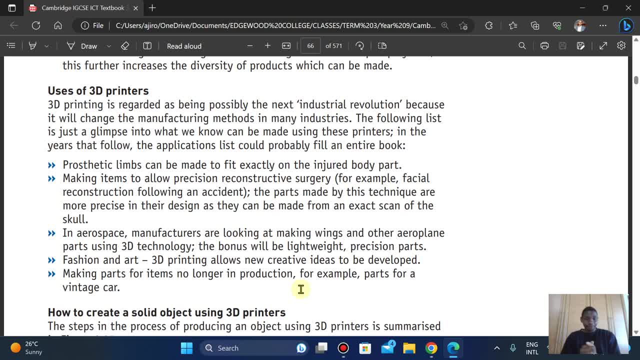 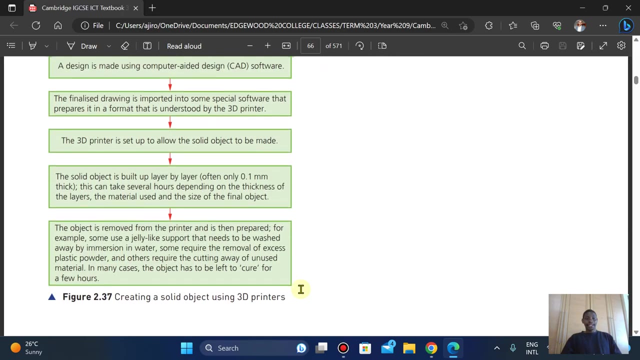 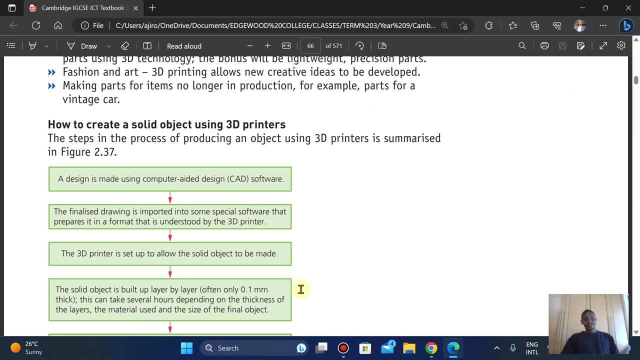 making items to allow position reconstructive surgery. manufacturing of parts of the set up skin case: ok, the bulunos will be lightweight. okay, position parts. making parts for items that no longer in production: right is very. 3d printers can actually do that- okay. and now there are steps on how a 3d printers can um be created. right, the design is made. using the computer aided design software. um the next one, it made the 3d printer, and so what it actually does is it? we use a 누�arfte Naturale do a 3d printer? um, and坐ing a 3d printer is pressure. 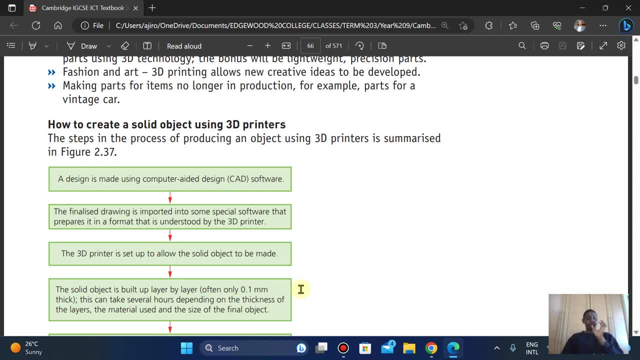 and I boiling it so that we have goodness. you can see the is the min SA Warrior now, but with a baby milk inside in black. so that means theé one is. the finalized drawing is imported into some special software that prepares in a format that's understood by the 3d printer. the 3d printer sets up to allow the solid objects to be made. 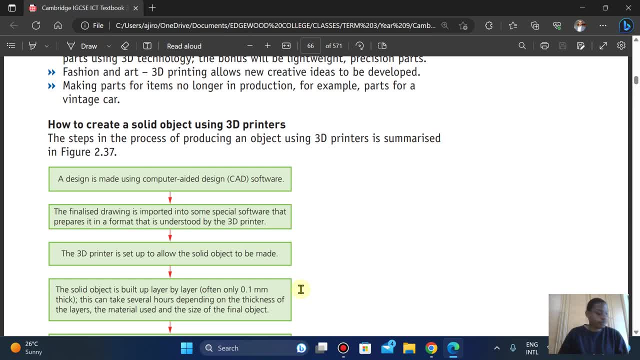 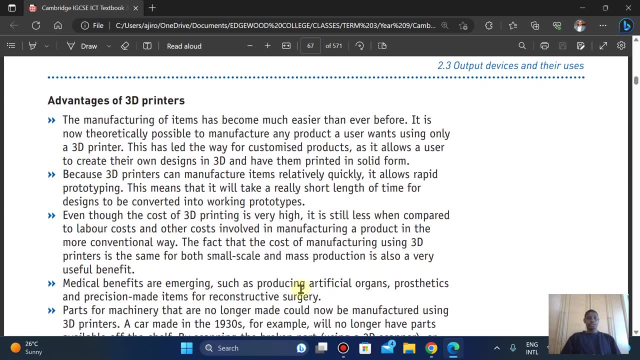 the solid object is built up layer by layer. okay, then, advantages of the 3d printers. let's talk about it. um, manufactures of item have become easier than before, okay. um, the 3d printer can manufacture item relatively quickly. um, even though the cost of the 3d printer is high, it is less when compared to labor cost. 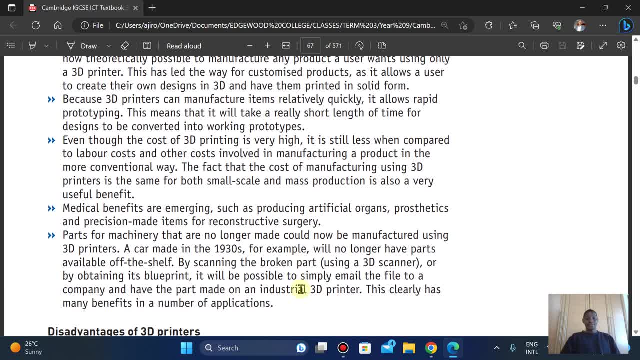 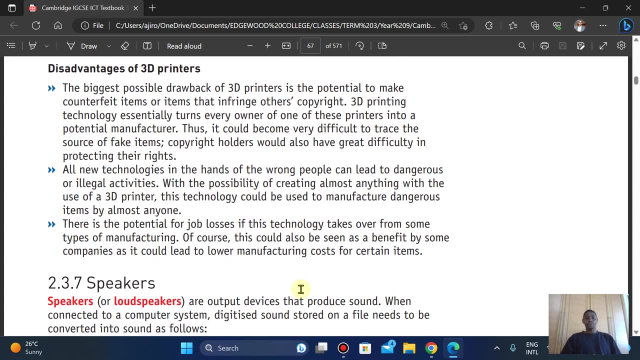 okay, um, medical benefits: i imagine prosthetic limb organs that can be used for that part of machineries are done. longer base cannot be manufactured using the 3d printers. okay, disadvantage is that the biggest possible drawback is that is, the potential to make a counterfeit item that infringes others. 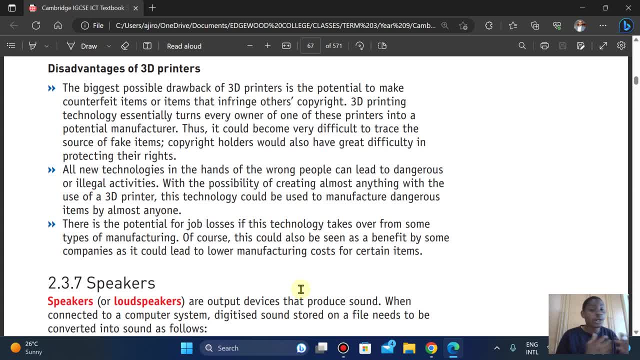 copyrights. now this is a possibility because you can make other items of people's design, even when you are not allowed to do that. okay, all technologies are now in the hands of the wrong people, which can be led to a dangerous or illegal activities. the 3d can actually produce. 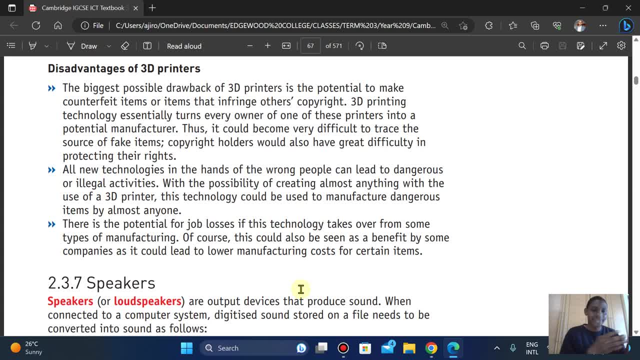 gone right and this cannot be detected with the um, the scans, and they can actually use it to harm people. now this: there's a potential of job losses if this technology takes over some type of manufacturing, because now it will be doing the work that um, um, the label, um humans will actually 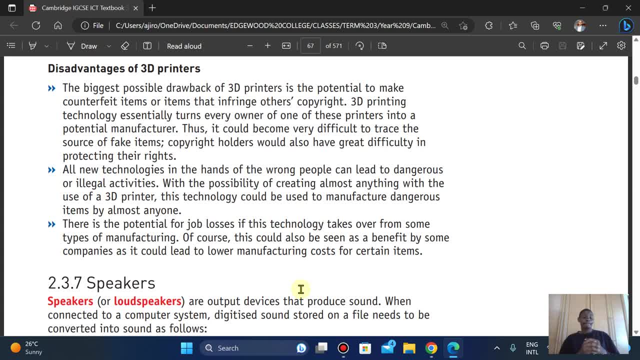 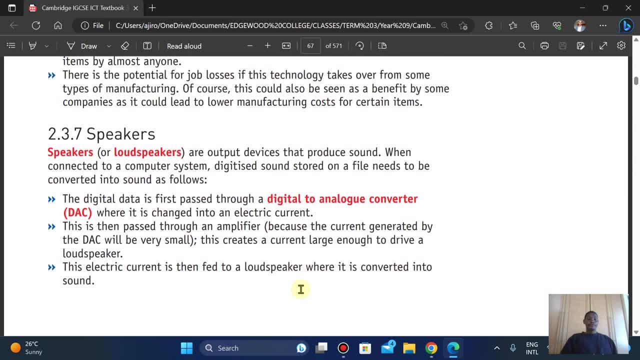 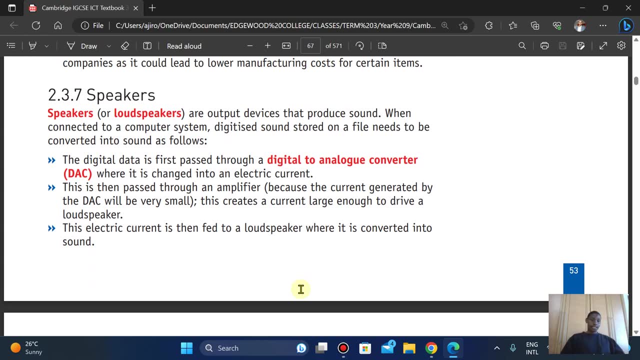 thereby um causing a form of unemployment. okay, um, let's talk about speakers, why speakers are used to produce sounds. okay, um, of course, obviously this is done with a dsc- that the digital data is first passed through the um dc and then it is changed to electric current, there is passed to 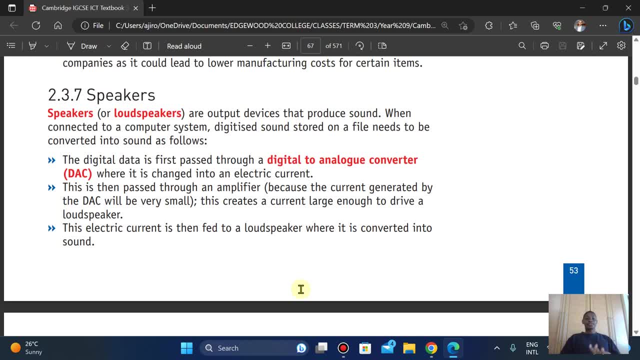 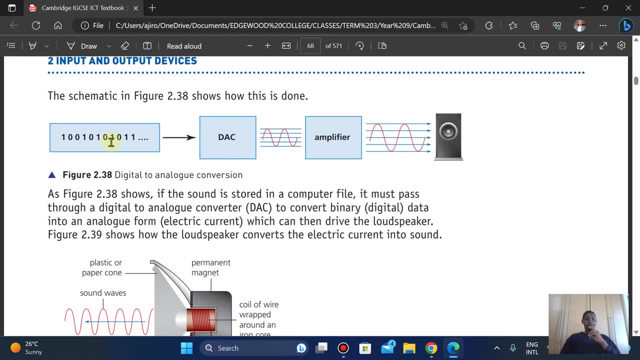 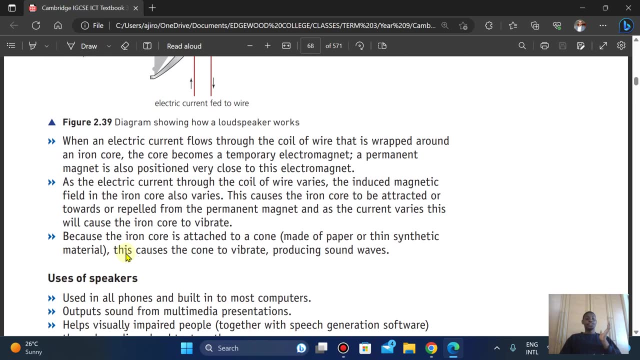 the amplifier and then it creates a large enough sound to drive to a last to loudspeaker etc, etc. right now you can see this is a bit the binary, but dc just gives amplifier and it goes to the speaker. now let's talk about the uses of speakers. they are using all phones. they are built in most computers. 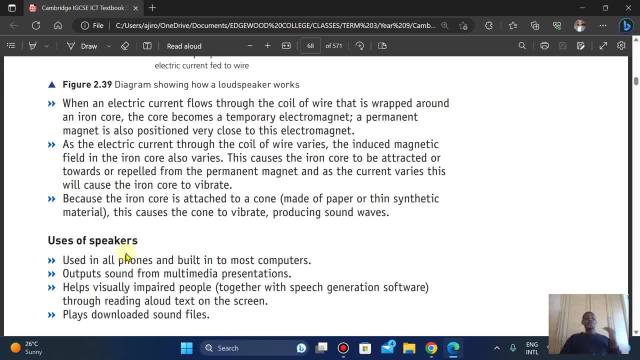 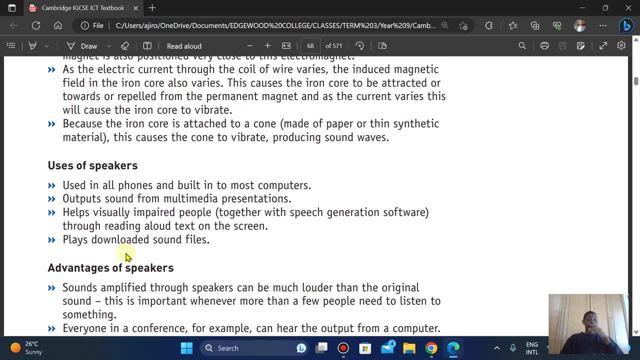 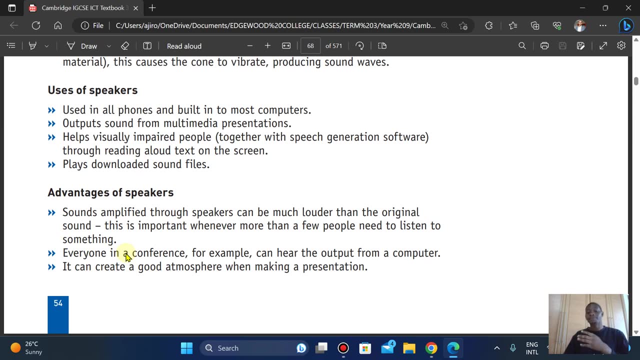 output sounds for multimedia presentations helps visually impaired people, okay, especially when you talk about speech generated softwares, um. play downloader sounds files, um. the next one is the advantages is the sound amplified. speakers can be much louder than the original sound, okay, which makes it easier for people to listen. okay, everyone in the conference is going to listen to. 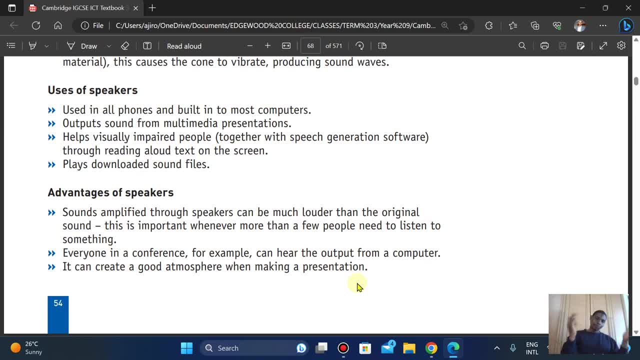 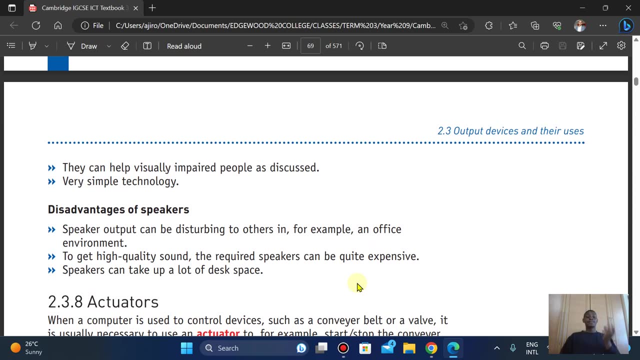 song. so if you listen from the computer, you can listen from the exposure of the computer. it can create an atmosphere when making a, a good atmosphere when you're making a presentation, because people can actually hear you from far. okay then, um, they can help visually impel people. 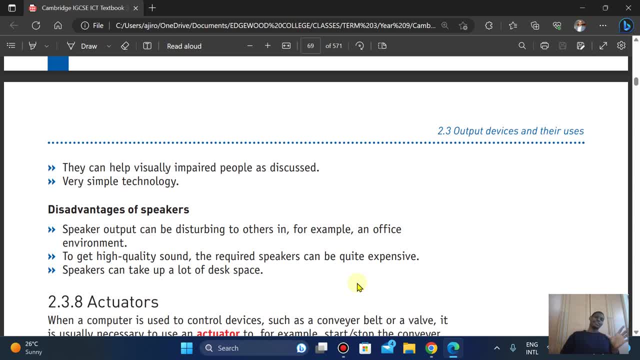 at this cost, right? um, it's a very simple technology, okay, speaker output can be disturbing to others, especially in an office environment. um, to get high quality sound, um, you need to be able to hear. you can actually hear the output from your computer. if you are playing an audio, it can be disturbing to others. 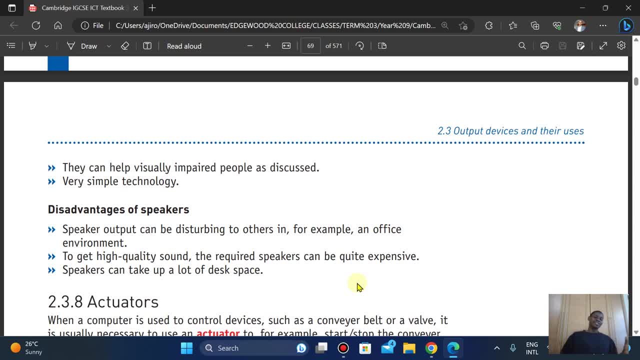 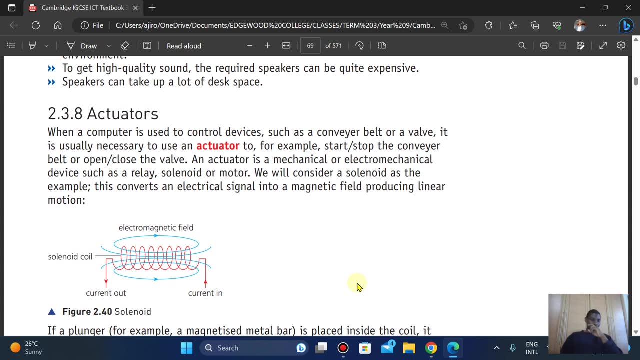 high quality sound, the required speaker can be quite expensive, right? If you're looking for a bass speakers speaker can take up a lot of the tech space because you have to buy them and put on your table, right? I think the last one is the attritus. Let's talk about them Now. attritus is 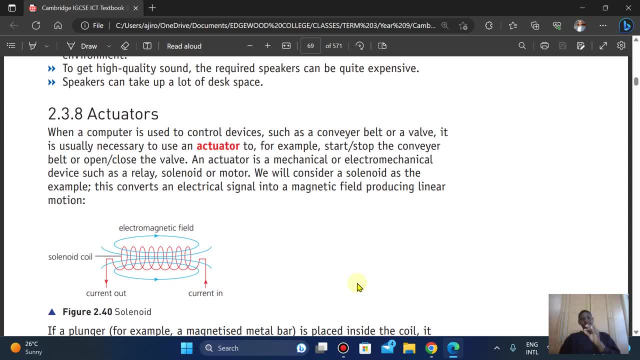 used to control devices. Now, when a computer is used to control devices such as a conveyor belt or a valve, it is necessary to use what we call an attritus. For example, it's a start and stop conveyor belt to open and close the valve. Now this attritus is a mechanical or a led to. 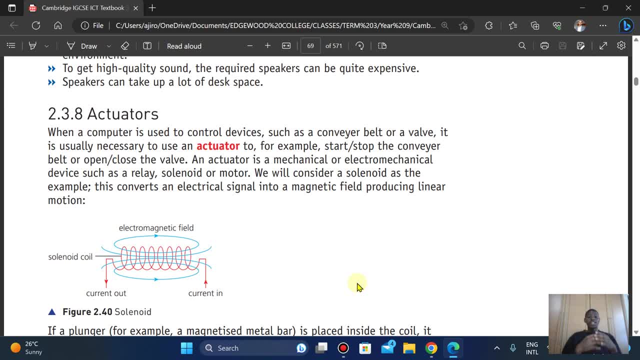 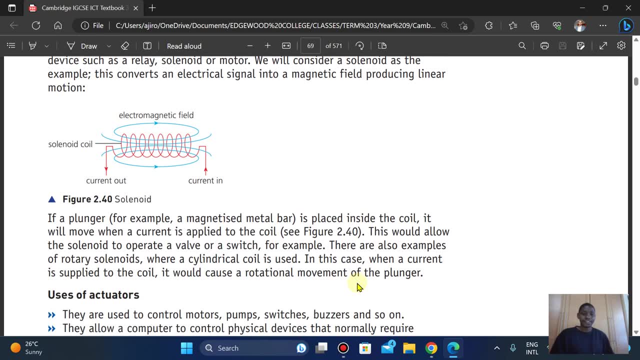 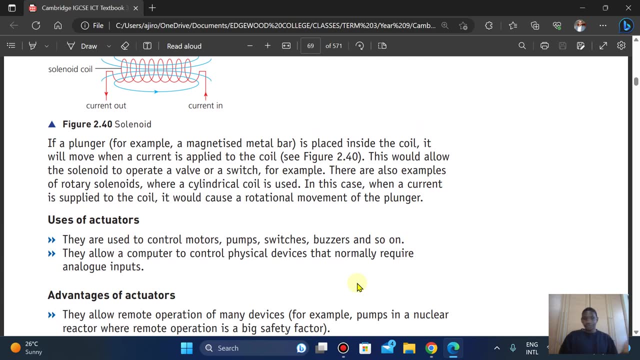 mechanical device such as a relay or a solenoid or a motor. Okay, What it simply means is it helps in movement. Okay, Now, attritus can be used to control motor Pumps, switches, buzzers, et cetera, et cetera. They allow a computer to control physical devices. 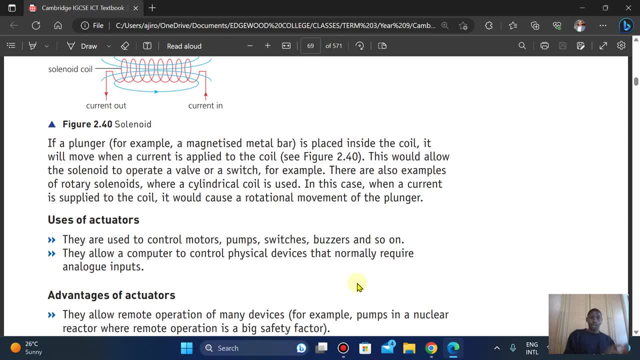 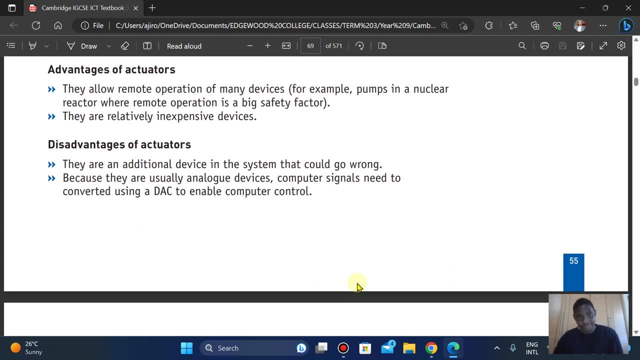 that normally require analog input. Okay, Now let's talk about the advantage of these attritus. They allow remote operations of many devices. Okay, Remote operations of many devices, For example, pumping a nuclear reactor, where remote operation is a big safety factor. They are really. 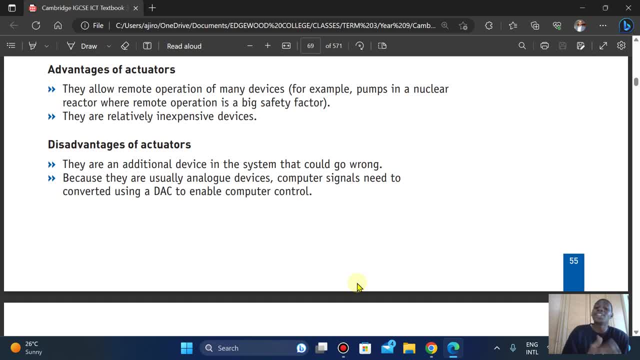 glitch-free and yet very risky. That is, they are relatively inexpensive devices. They're not quite as expensive and easier to build up. Okay, Now, the disadvantage is that they are additional devices in the software that could go wrong, especially if you're conveying that device. 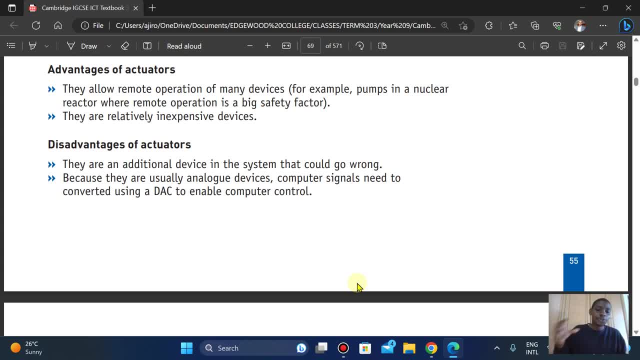 signal to the attritus that you built that is not responding. Because they usually are analog devices. computer signals need to be converted. Remember this are analog device. right, because An action Okay. so the computer signals need to be converted using what we call a DAC, digital analog converter. 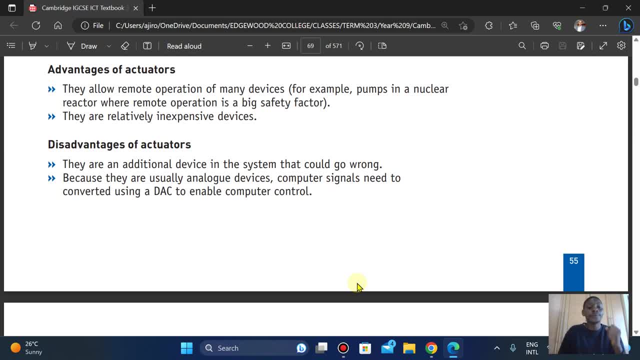 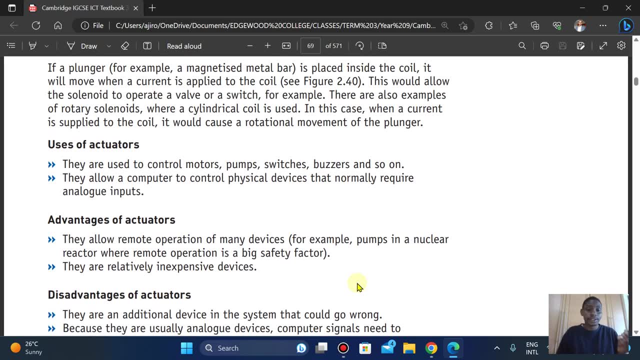 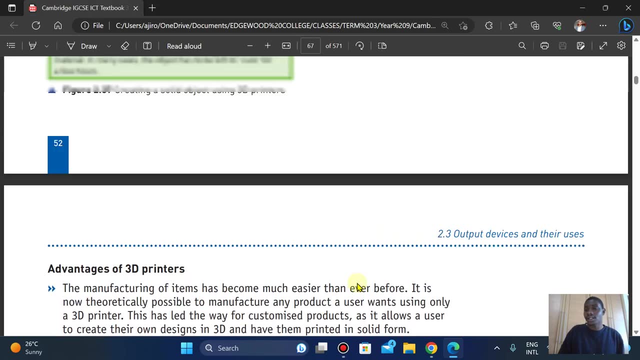 to enable the computer to control these Actuators. Okay, so that's all about our two devices We've talked about. We started with the monitor screens and then, for the monitor screens, We talked about the CLT, the LCDs, the LEDs, Okay, and then we moved over to 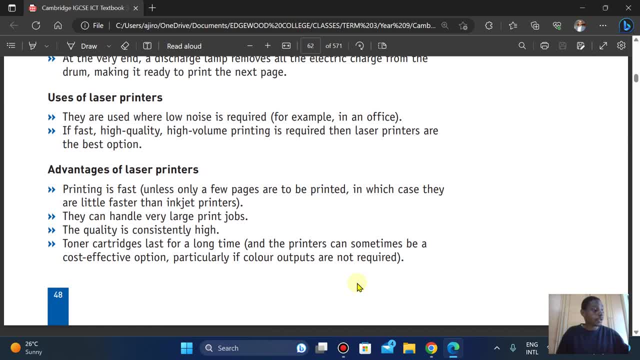 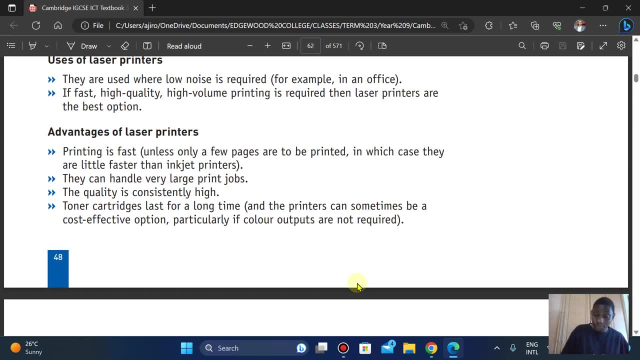 Printers. So touch screens: we talk about touch screens as the output devices. We'll talk about touch screens as an output devices, Which is based on the previously imputes, and then we'll talk about printers, which is the inkjet, the laser jets, Then the touch matches, and they will talk about the 3d inkjet printers and then we moved over to the plotters. 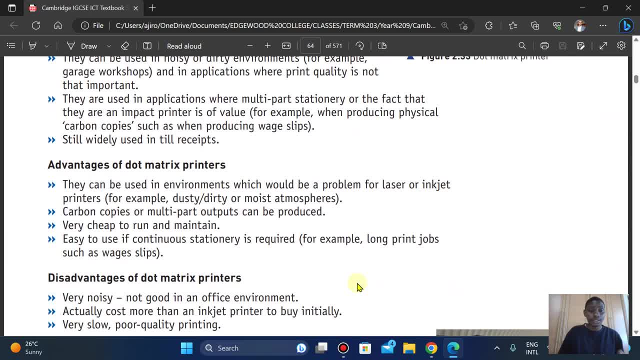 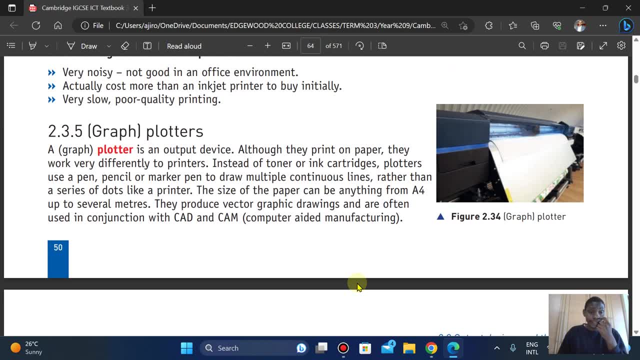 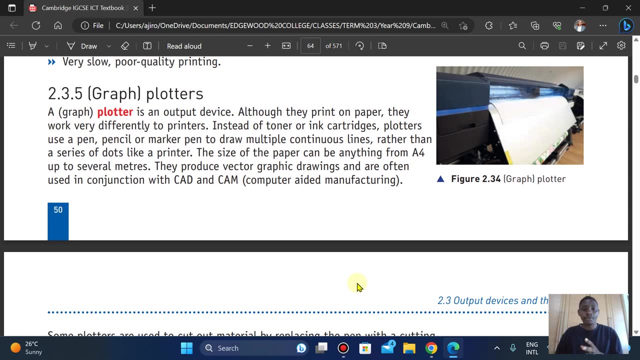 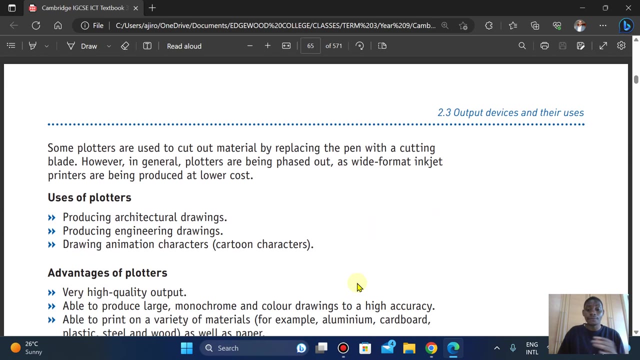 Right. that makes it of either a pen, A pen pencil, to actually draw on it, right. and and another beauty about the plotter is Or a marker right- is that it can draw not just on a4, but it could be used to draw on Aluminum, cardboard or anything plastic right. 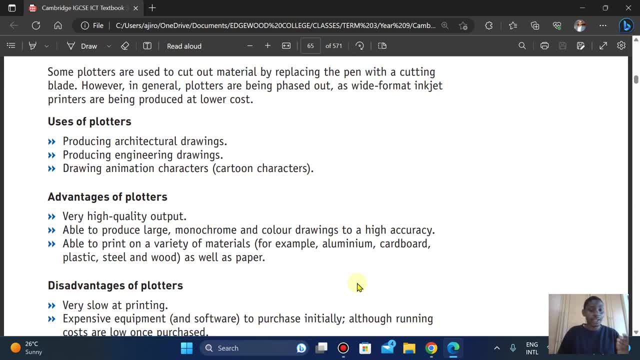 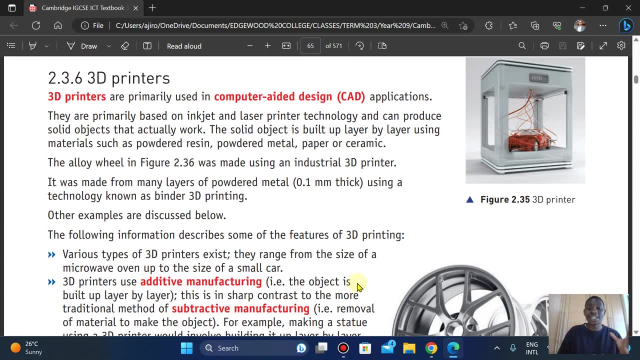 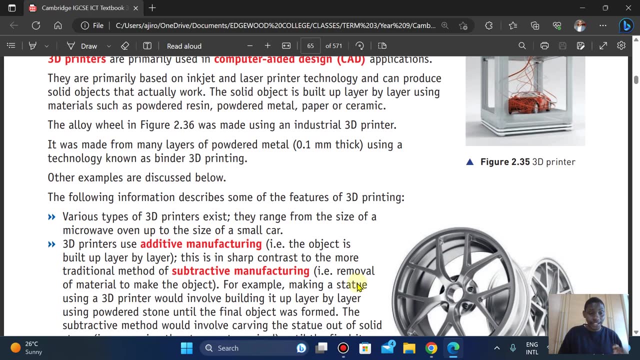 Still wood to draw on it. Okay, and we talked about the 3d printer, which are used to produce solid objects that we work it prototype Whenever you can imagine it produces, and this is done by its software called the computer in the design. We should now sent to the 3d printer to get this done and 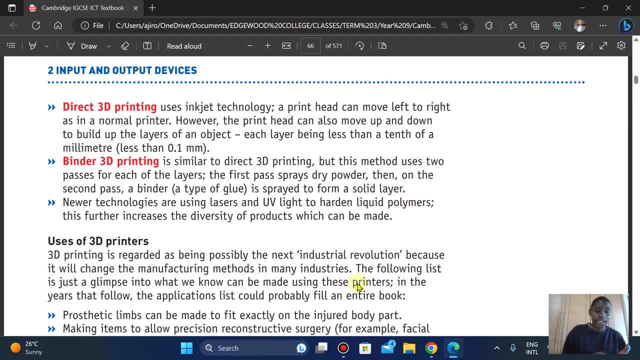 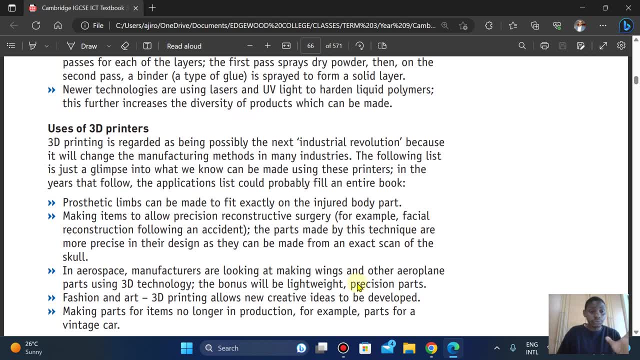 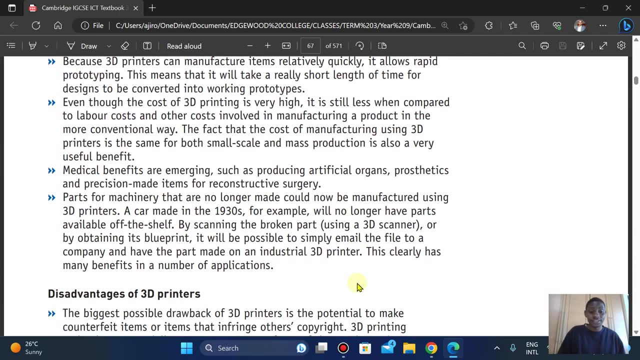 We've looked at the advantages of how it can be applied in so many industries: for your hospitals, For the medical, medical manufacturing, etc. etc. and then we looked at how to create it and then we'll look at its advantages. what we talked about um the fact that it could be in the wrong hands and they gave you to produce something dangerous. 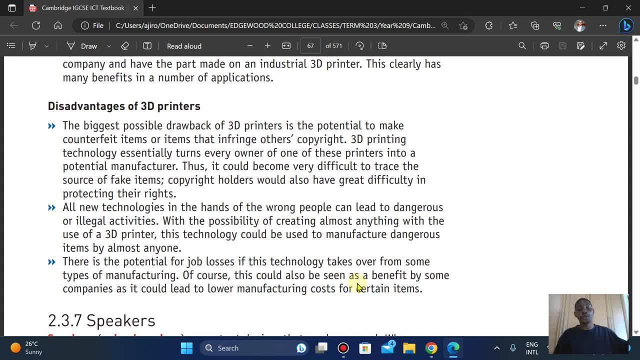 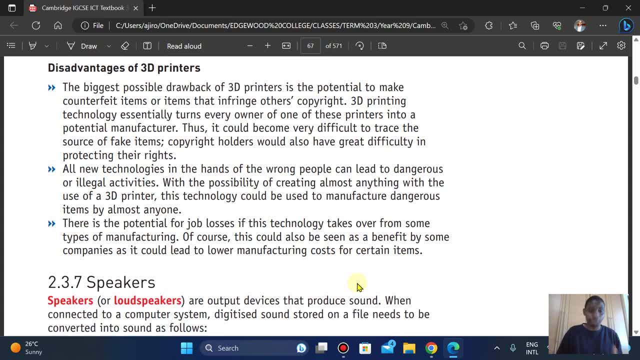 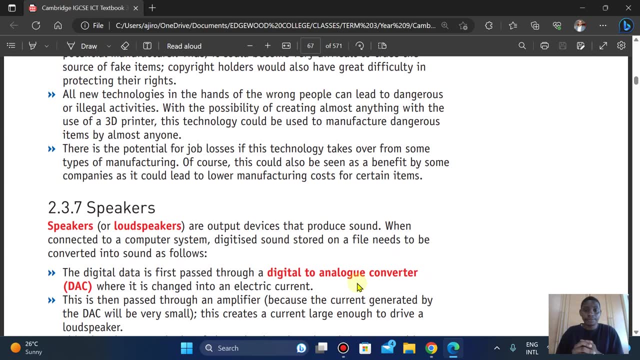 in liga and we look at um. the drawback is, people can actually use it to make um items of things that they don't have authorization for, okay, and we also look the fact that if it's been applied to other technologies, um, people might actually lose their job. and then we talked about speakers. 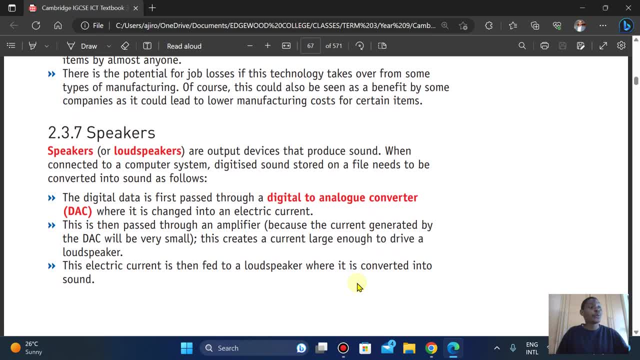 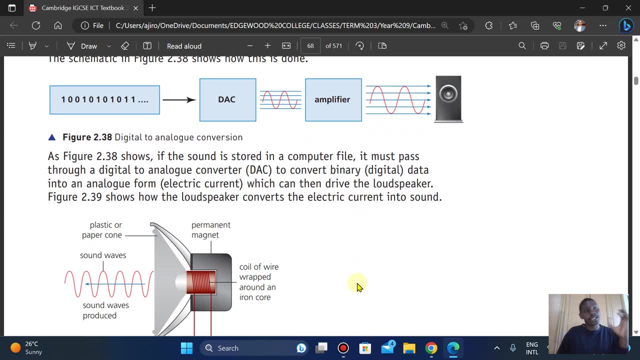 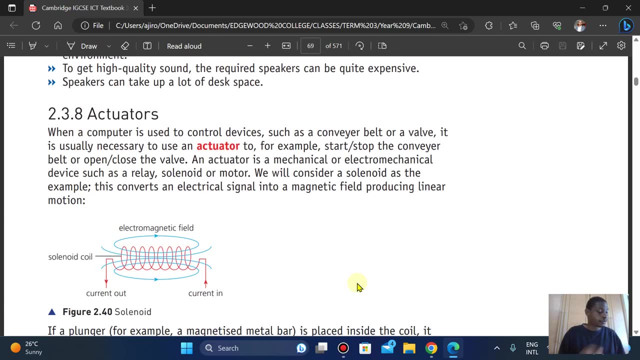 and we said we talked about digital to analog converter, where it is now changed to electric current, and then we um we talked about the uses that it helps to amplify our voices and um we talked about attritus, which is more like a mechanical device that helps to um control. 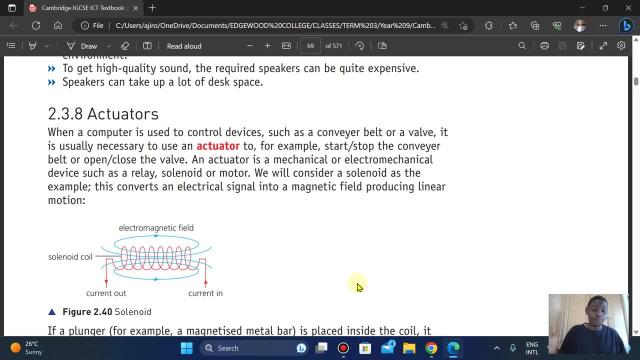 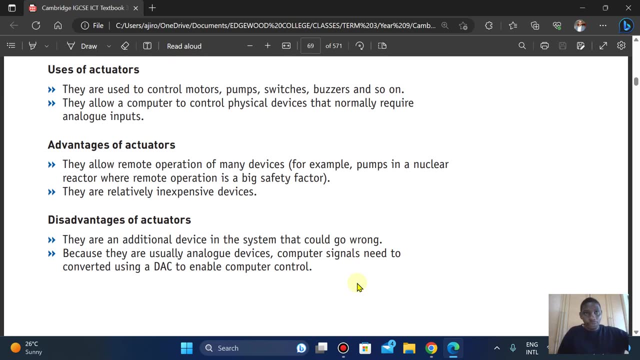 right. so, um, and then talked about that is not expensive to build and as much as possible. whenever this is um, we talked about disadvantage. where we talked about that, um, we could have issues when it's not responsive. what do we mean is, simply, if the computer is not able to send the signals to it and um, most of the